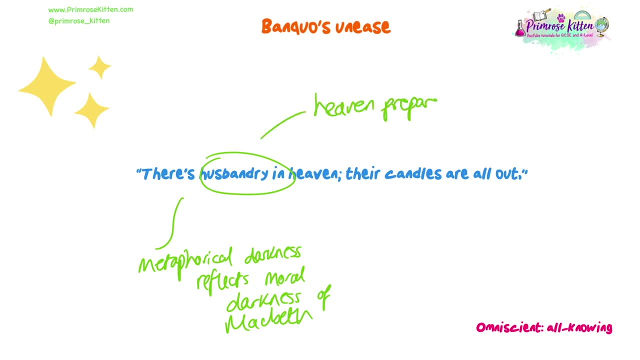 king's impending doom. This observation subtly recalls earlier instances where Macbeth and Lady Macbeth called upon darkness to mask their deeds, reinforcing the theme of appearance versus reality. For a Jacobean audience, this darkness would also imply the inescapability of divine judgment. 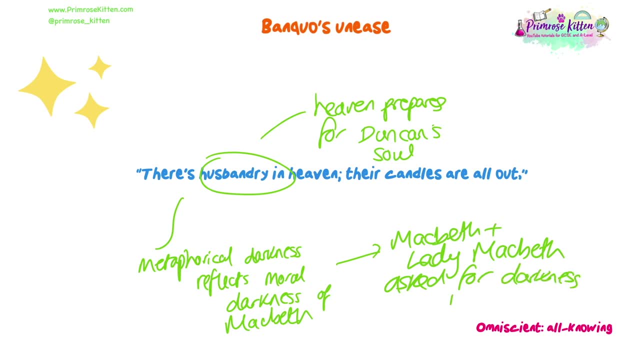 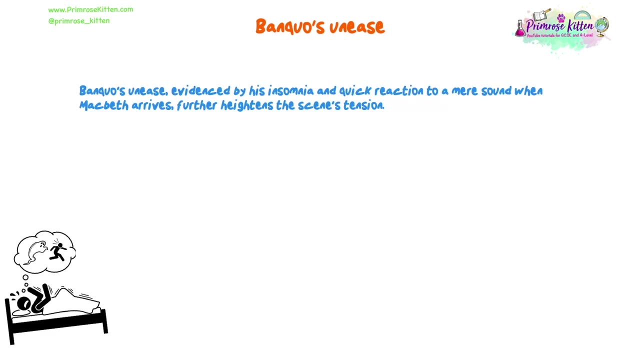 suggesting that no sin, especially regicide, can be hidden from God's omniscient gaze. Banquo's unease, evidenced by his insomnia- quick reaction to a mere sound, even when Macbeth arrives, further heightens the scene's tension. 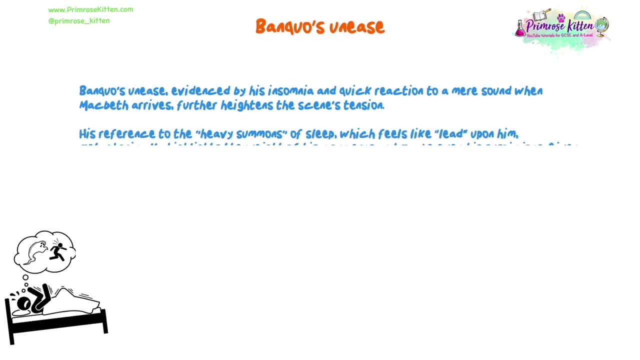 His reference to the heavy summons of sleep which feels like lead upon him metaphorically highlights the weight of his concerns and maybe even his suspicions, Given his knowledge of the witch's prophecies. Banquo's wariness around Macbeth could be read as early signs of suspicion or, at the very least, a deep-rooted unease. 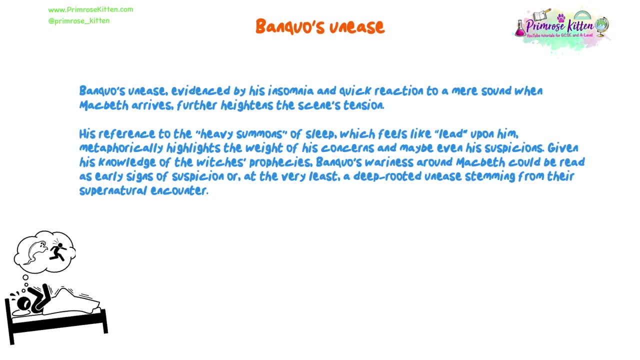 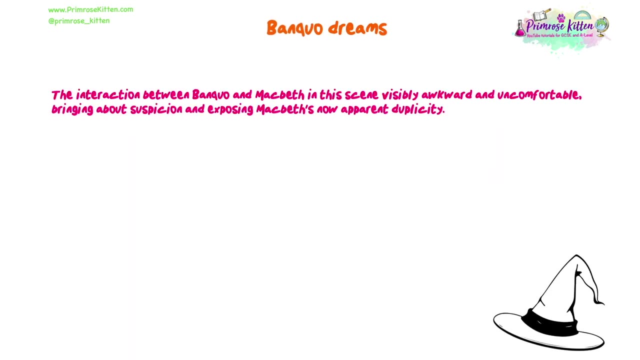 stemming from their supernatural encounter. The Jacobean belief that demons were responsible for troubling dreams aligns with the notion that the witches have indeed sown the seeds of chaos and corruption, influencing the natural order and the character's mental states. The interaction between Banquo and Macbeth in this scene is visibly awkward and uncomfortable. 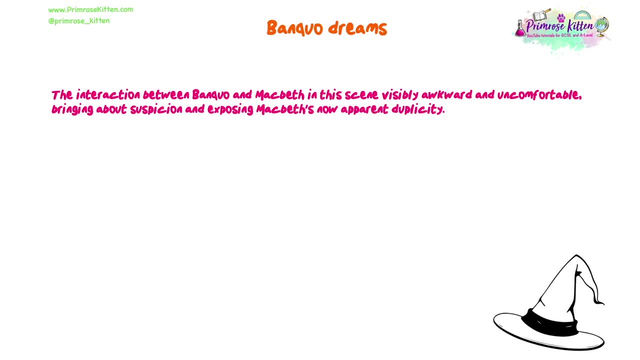 It brings about suspicion and exposes Macbeth's now apparent duplicity, and if you are duplicitous, it just means you are two-faced. Banquo's reference to his dreams of the, the three weird sisters, and their partial truthfulness to Macbeth, serves multiple purposes. 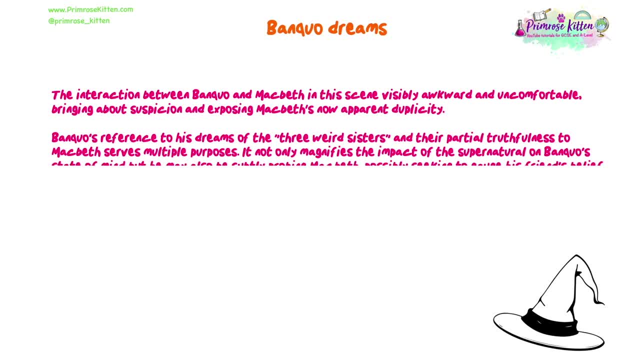 It doesn't only magnify the impact of the supernatural on Banquo and his state of mind, but it might also be subtly probing Macbeth too. He might be seeking to gauge his friend's belief in the prophecies or his ambitions For a Jacobean audience. like we said before, they were familiar. 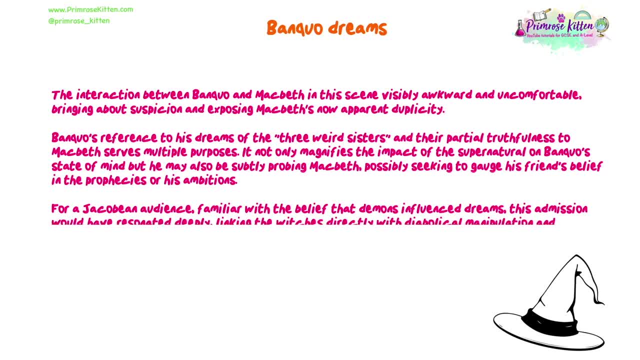 with the belief that demons influence dreams. so him having this conversation with Macbeth would have resonated deeply with the audience, linking the witches directly with manipulation and, as we said, it foreshadows the chaos they've unleashed upon the natural and moral order in Scotland. Now Macbeth's response to Banquo is telling as well. his offer of honour to Banquo. 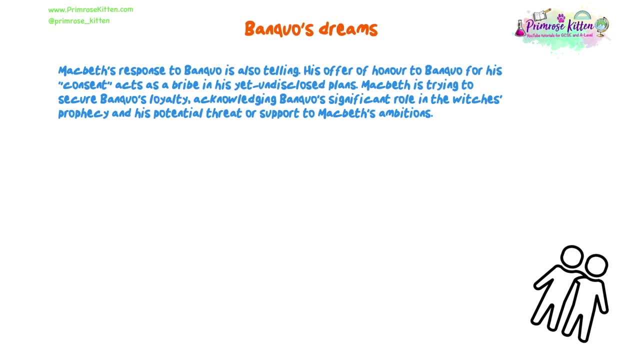 for his consent acts as a bribe. in his yet undisclosed plans, Macbeth is actually just trying to secure Banquo's loyalty. acknowledging Banquo's significant role in the witches prophecy and his potential threat or support to Macbeth's ambitions At present, don't forget. 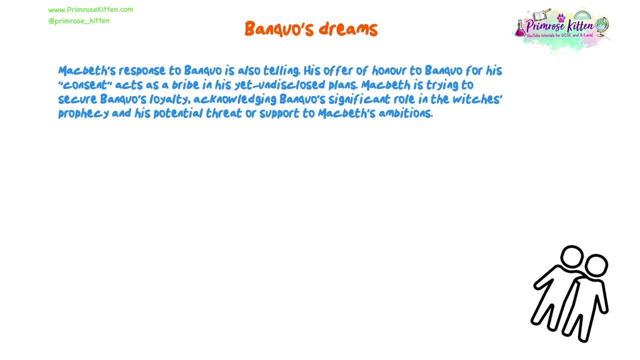 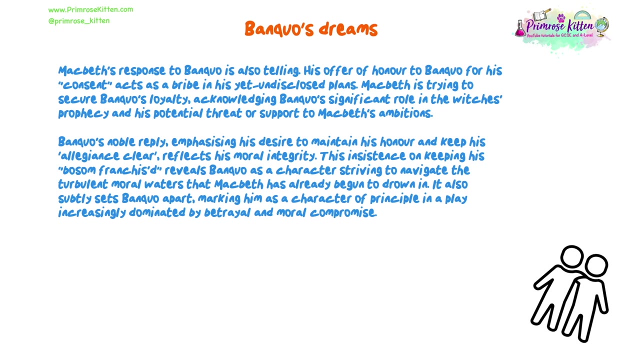 Banquo is the only one that has reason to be suspicious, because if anything happens to Duncan at this castle, then it's going to look likely from Banquo's perspective that Macbeth did it because he would have reason to after what the witches said to him. Now, when Macbeth makes this, 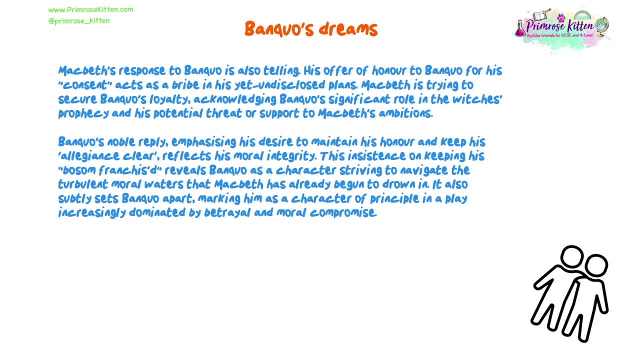 offer and he makes this bribe. Banquo's noble reply emphasises the fact that Banquo is a his desire to maintain his honour and keep his allegiance clear, and it reflects his moral integrity. He says so. I lose none in seeking to augment it, but still keep my bosom franchise and 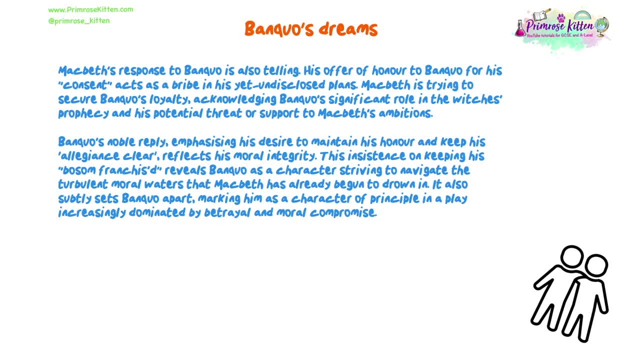 allegiance clear, I shall be counselled. He essentially says. so long as he can keep his conscience clear, he is happy with Macbeth's offer. Now, this insistence on keeping his bosom franchised reveals Banquo as a character striving to navigate the turn of the world. 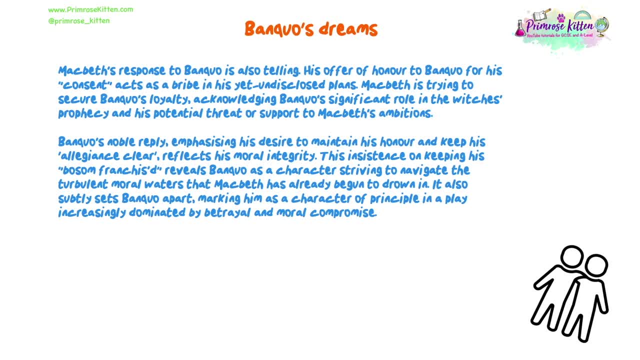 Perbulant moral waters that Macbeth has already begun to drown in. It also subtly sets Banquo apart, marking him as a character of principle in a play increasingly dominated by betrayal and moral compromise. So this is really where you start to see the difference between Banquo and Macbeth. 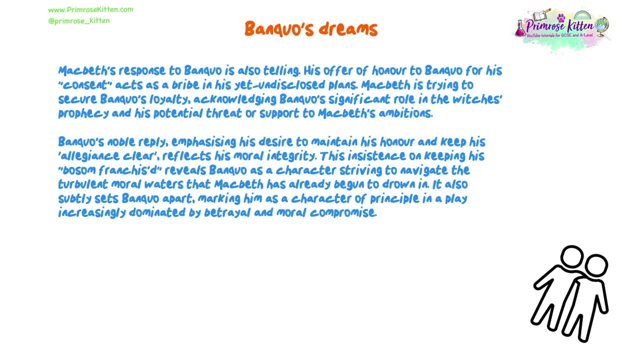 because where Macbeth has already sort of fallen into this trap and falling victim to his hamasha, Banquo is not the same. So what we could say is that Banquo is a foil to Macbeth, and a foil is a character that completely contrasts another, with the purpose of 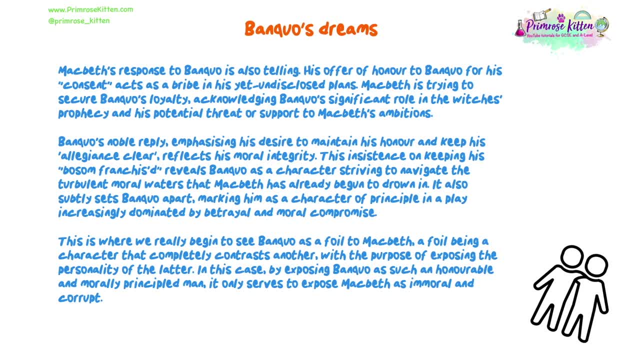 exposing the personality of the latter. So, as an example, in this case, by exposing Banquo as such an honourable and morally principled man, it only serves to expose Macbeth as even more immoral and corrupt, because they are so, so different. Now, this dialogue is absolutely full of tension. 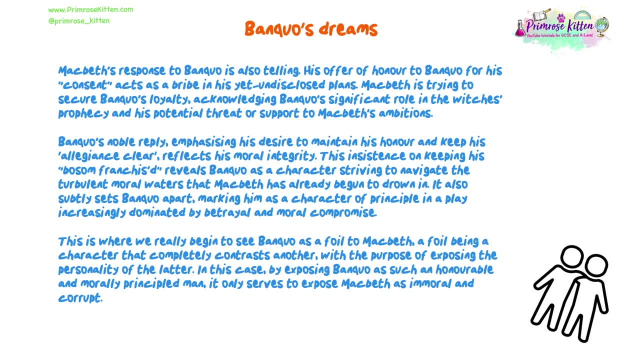 and ambiguity. It's a real clever depiction of the shifting of power dynamics and loyalties that characterise Macbeth. where we would have maybe once considered Macbeth and Banquo as the best of friends, We now see that he is paranoid, concerned about Banquo and Banquo is slightly, potentially a little bit. 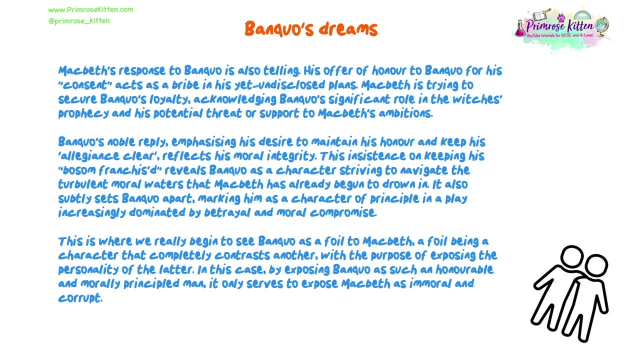 worried about him as well. So for the audience, this interaction really heightens the suspense leading up to Duncan's murder and it deepens the tragedy of Macbeth's transformation, Because he was once considered this noble warrior and he's now becoming this tyrannical murderer. 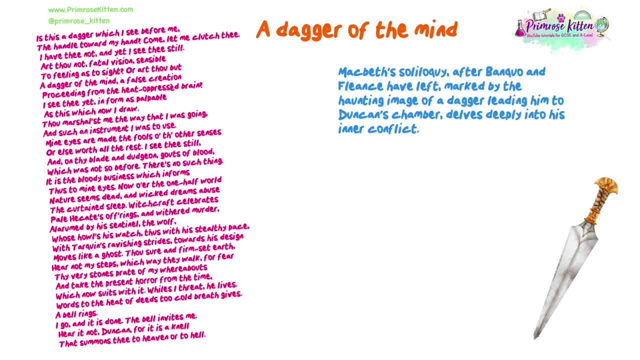 Now moving on to the soliloquy. we've got Macbeth's soliloquy, really, really famous one, and it's after Banquo and Florence have left. don't forget: soliloquies are spoken to the audience while the character is alone on stage. It marks the haunting image of a dagger. 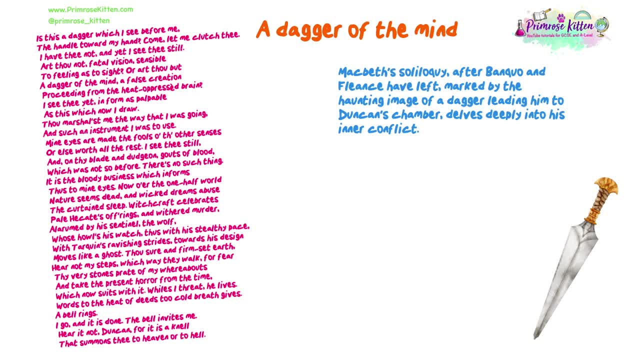 which leads him to Duncan's chamber or his bedroom. It delves deeply into his inner conflict. The dagger of the mind signifies Macbeth's internal conflict and guilt. it serves almost as a harbinger or a sign of the bloodshed that's coming. 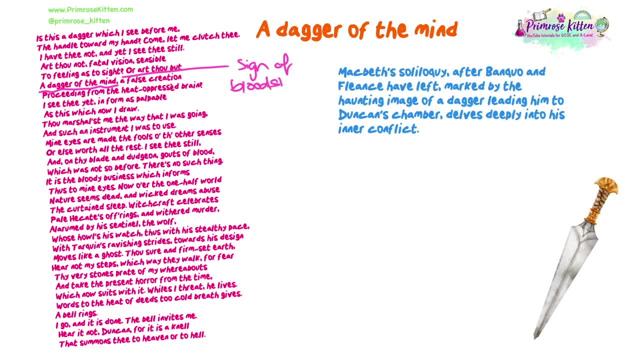 His questioning of the dagger's reality. he says things like: are not fatal? vision sensible to feeling. as to sight, it reveals his growing instability. He's a man on the brink of committing an act so sinful it disturbs the very fabric of his being. 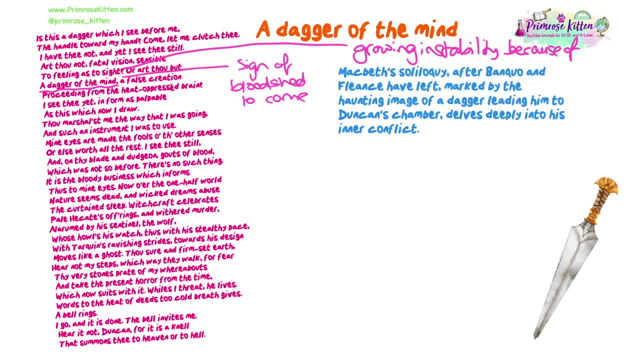 Here he actually has to challenge and question himself to ensure he can keep hold of his sanity. You'll see there's lots and lots of questions and lots and lots of question marks in that part of the soliloquy. He also questions whether the hallucination comes from a heat-impressed brain. 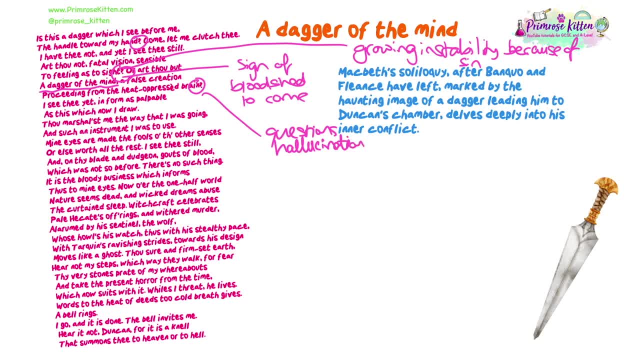 so essentially he's asking whether this hallucination that he's seeing is because of a fever or an illness. Now, that's interesting because it kind of metaphorically aligns Macbeth's murderous intentions with illness, disease or, like we say, fever. It kind of suggests that his 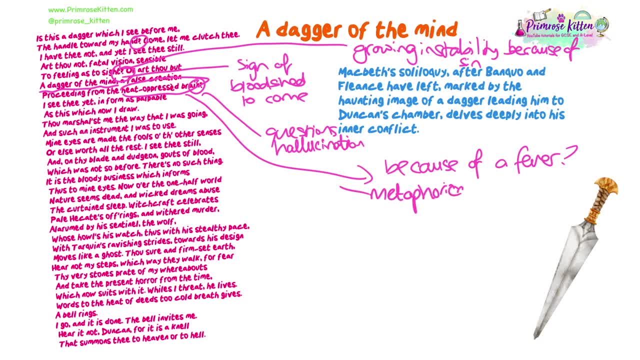 moral corruption has induced or created a state of delirium. He's delirious. in other words, The word heat actually implies pain and suffering, so that's a really good thing to kind of zoom in on. And when coupled with the word oppressed, that means being subjected to cruel treatment. 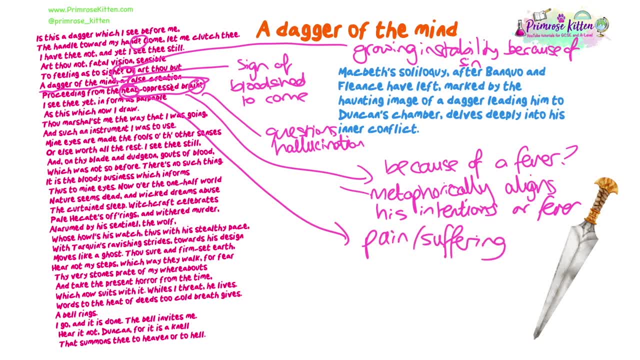 usually for long periods of time. It implies that the suffering is becoming inescapable, like oppression would feel, And it foreshadows the permanent suffering of damnation he will experience following the murder as well. So there's lots of methods you can look at with that quote. 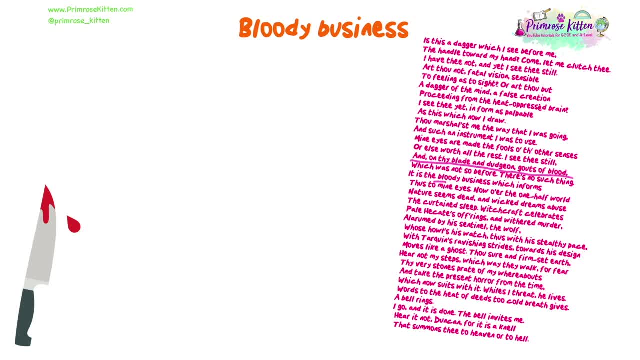 The soliloquy progresses into visions of blood on the dagger and it underscores the inevitability of guilt staining the Macbeths. That's Macbeth and Lady Macbeth, because that's their surname. It's a potent or powerful foreshadowing of Lady Macbeth's later descent into madness, Don't forget. 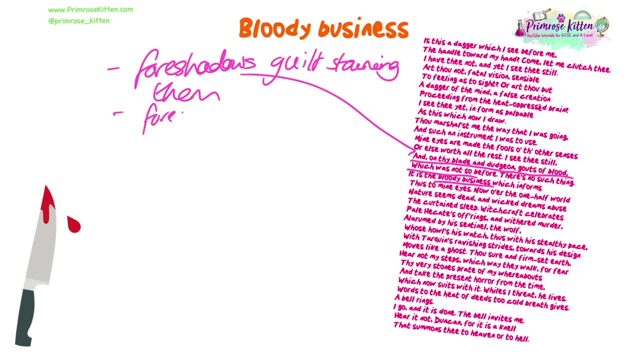 in Act 5, Scene 1, she attempts to wash away imagined blood from her hands. It almost foreshadows that moment. Macbeth's acknowledgement that the bloody business as well informs these hallucinations underscores his awareness of the moral and psychological ramifications. or 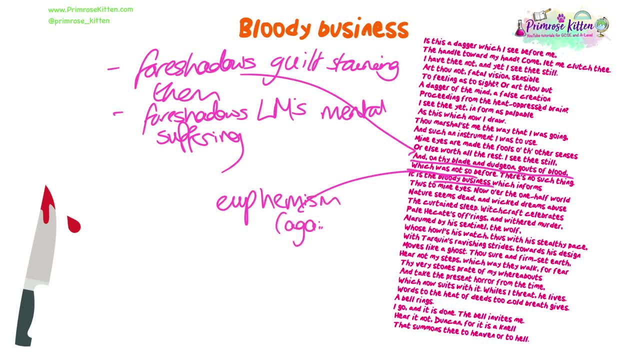 consequences of his actions. He repeatedly uses euphemistic language like this to comment on the murder. This isn't the first time we've talked about euphemism And it again proves his naive attempt to rid himself of the murder. And it's a potent or powerful foreshadowing of Lady Macbeth's. 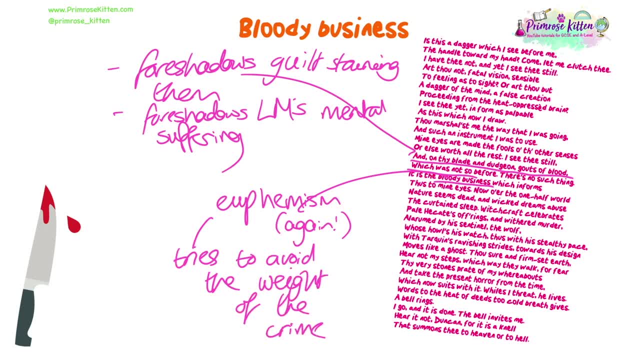 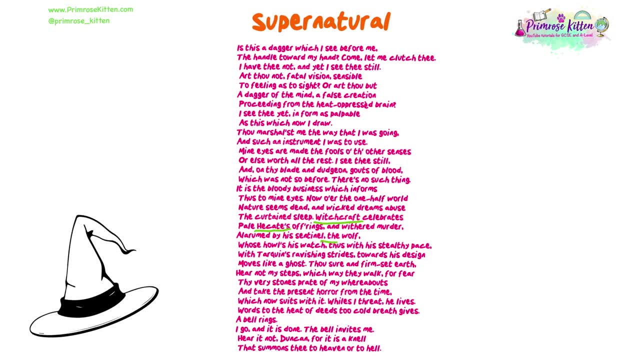 gravity of his crimes. Then later in the soliloquy, the supernatural undertones intensify because Macbeth, he mentions witchcraft with Hecate, the goddess of the witches, and other dark entities. There's the word ghost, there's the word horror, for example, 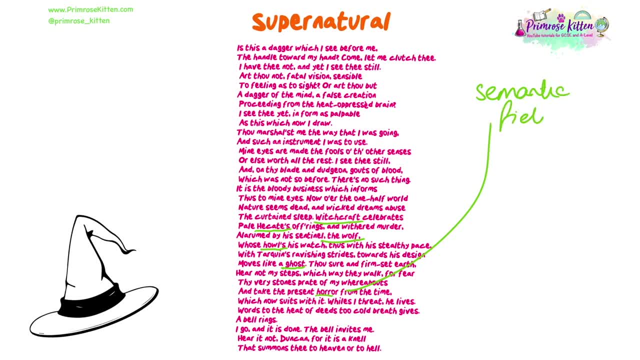 He really reflects his entanglement, his mental entanglement, with forces of evil, And by entangled I just mean when he met the witches, he's become really, really gripped by them And he's now tangled up in the forces of evil. And he's now entangled in the forces of evil And he's now 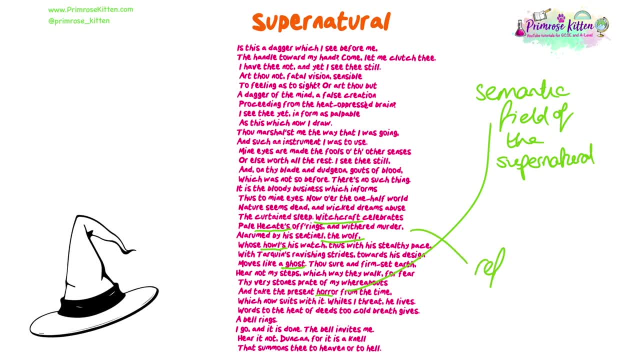 in this world of mental instability and turmoil. because of them, And then because we've got loads of words linked to the same thing, we can call that a semantic field. They're all linked to the supernatural. So this semantic field not only illustrates Macbeth's downfall, but it also 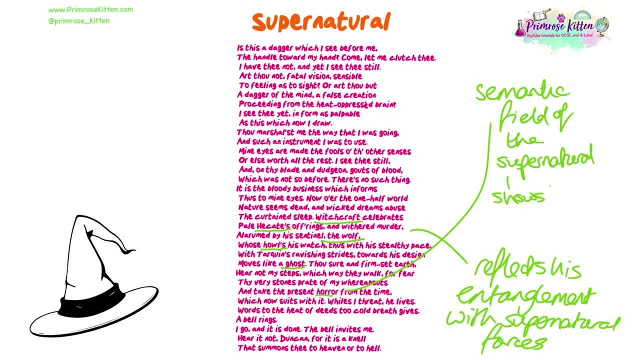 aligns his fate with the chaos and disorder that was started by the witches, reinforcing the play's exploration of supernatural influence on human actions. Because, don't forget, his audience at the time would have been fascinated with witchcraft and the hysteria surrounding it was huge, Don't. 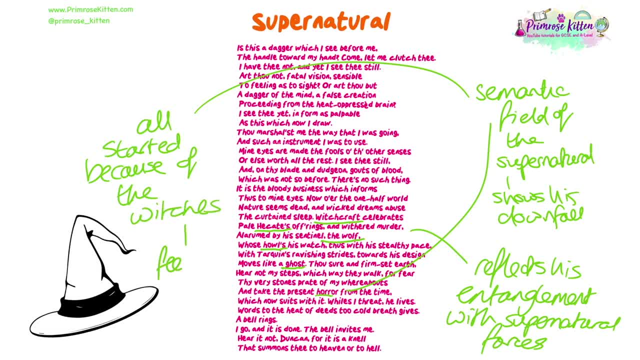 forget King James was so interested he wrote a whole book on it. So to feed the audience's fascination like this would have sparked fear and curiosity. I suppose you almost want to imagine it as sort of common things that people are scared of today If they were put onto a TV show or a film. 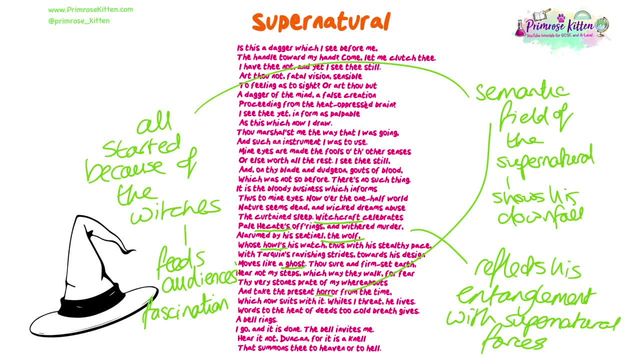 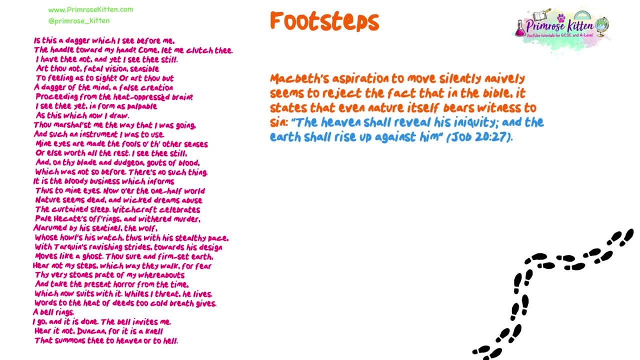 think about things that you guys are scared of. You might want to watch out of curiosity, but it kind of adds to your fears as well, doesn't it? Macbeth's aspiration to move silently, hoping thy very stones break, not on my whereabouts. 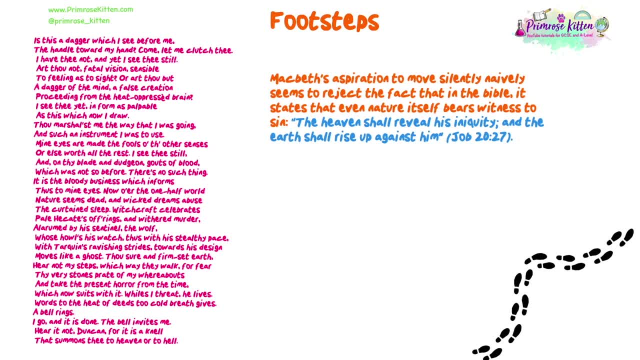 naively seems to reject the fact that in the Bible it states that even nature itself bears witness to sin. In the Bible it says: the heaven shall reveal his iniquity and the earth shall rise up against him. So in this case it should serve as a reminder to Macbeth that even 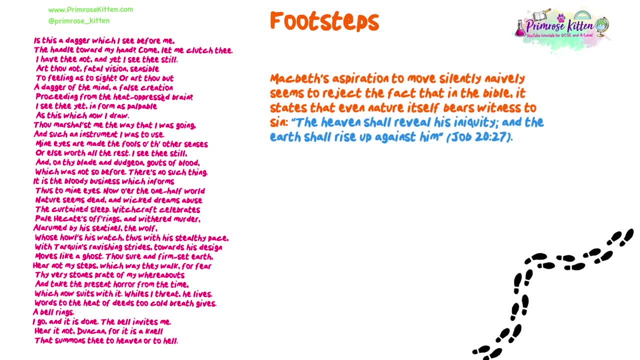 the earth sees what he has done. He can't escape God's judgment. He can't escape his own actions. The fact that he wants to be so quiet reveals his deep-seated paranoia. And he does actually recognise the natural order's retaliation against regicide. Even the natural world will reject what. 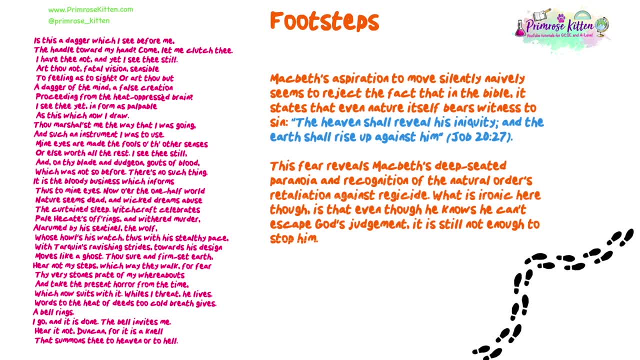 he's going to do. But what's ironic, though, is that even though he knows he can't escape God's judgment again, it's still not enough to actually stop him doing it. How the soliloquy and the scene ends with the ringing of a bell, it encapsulates his tragic 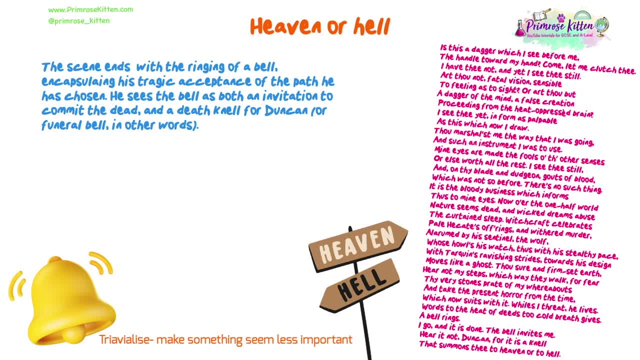 end. He's not going to be able to escape God's judgment. He's not going to be able to escape acceptance of the path he's chosen. He sees the bell as both an invitation to commit the deed and a death knell for Duncan. And knell is just a funeral bell, So it reveals the duality or 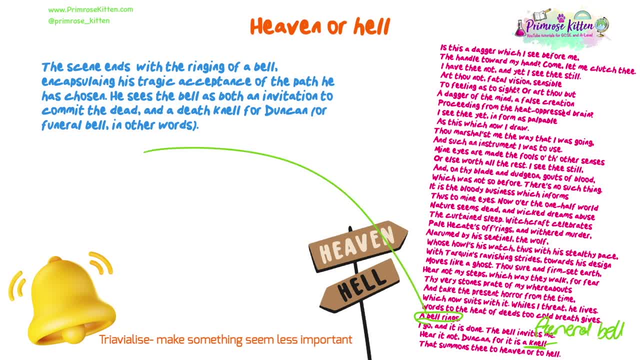 two-sidedness, in other words, of Macbeth's actions. On the one hand it ushers him towards kingship, But on the other hand it seals his damnation. Now, the idea that this bell summons Duncan to heaven or to hell is actually quite strange. 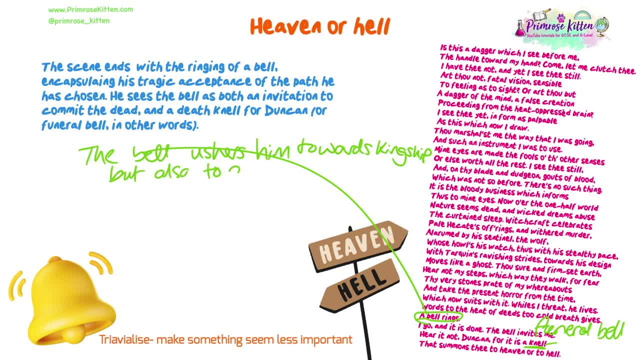 And this again is because we know that Jacobean's, due to the divine right of kings, believe that the king would go to heaven due to being chosen by God. So Macbeth suggesting he may also be sent to hell is strange. It might actually just reflect Macbeth's desperate and 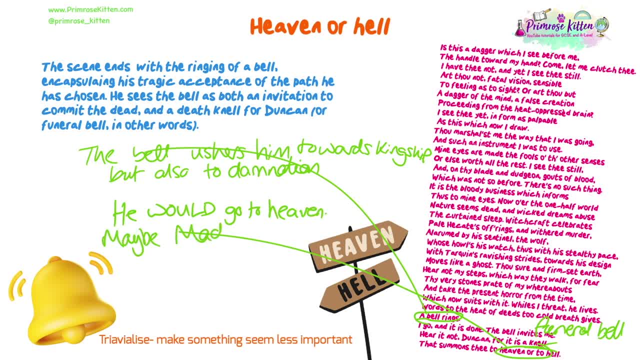 almost delusional attempt to rationalise or even trivialise the act of regicide. He's trying to kind of minimise it, so maybe it hurts him less, But it's actually quite blasphemous to assume that he would be deserving of hell as well. 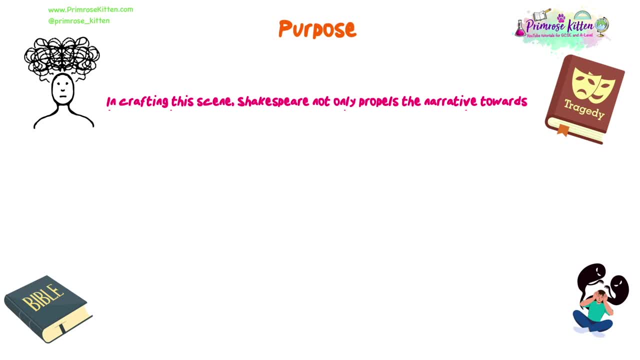 So think about purpose, then. When Shakespeare crafts this scene, he's not only propelling the narrative towards its dark climax, but it also deeply engages with the Jacobean audience's many anxieties around regicide, the supernatural and divine judgment. Ultimately, it serves to support 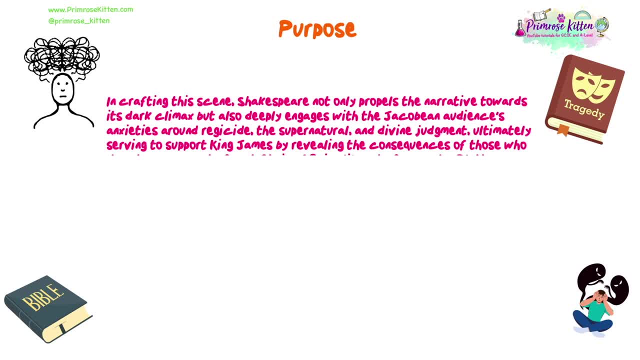 King James in that sense, because it reveals the consequences of those who dare transgress the great world, being like the gunpowder plotters attempted to do So. there's lots of interests and fears being addressed in this play, and then this scene in particular. It's very, very cleverly put. 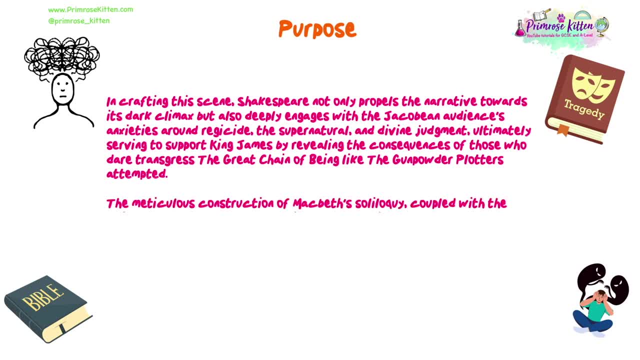 together. So this meticulous and careful construction of the soliloquy, coupled with that really horrible and ominous atmosphere, serves to heighten the tension and expose the play's tragic trajectory. It's marking a pivotal moment where the natural order within Scotland begins to unravel. 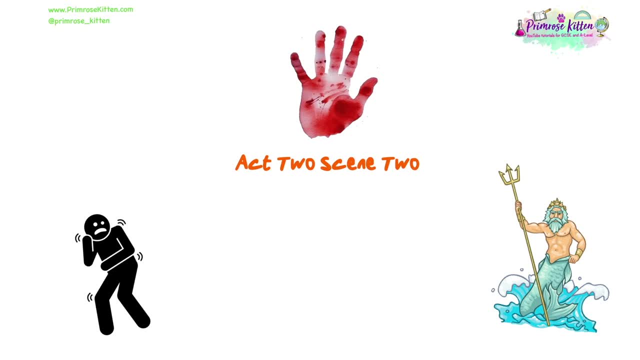 Act 2, scene 2 of Shakespeare's Macbeth plunges the audience into the immediate aftermath of Duncan's murder. It's a pivotal moment that, of course, alters the course of the play and its characters. This scene explores psychological turmoil, moral conflict and supernatural. 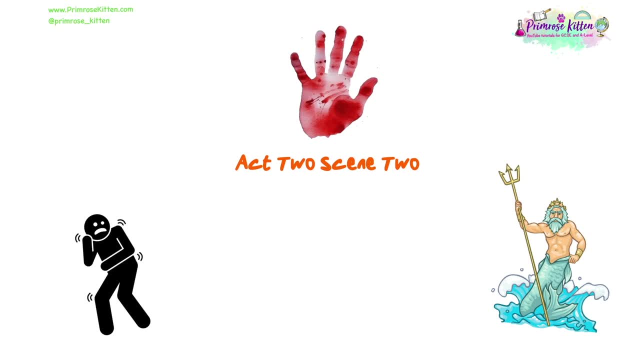 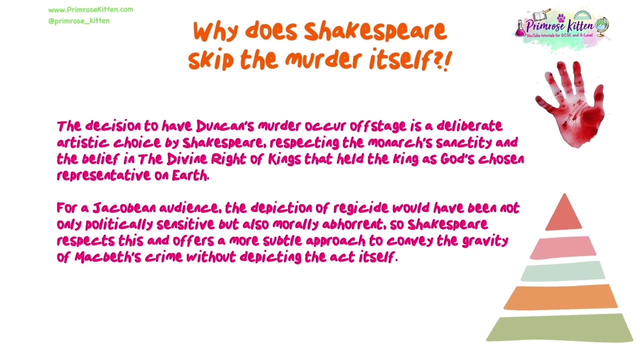 influence and it's displayed through Shakespeare's use of language, biblical illusion and the exploration of Jacobean themes such as divine right and regicide's damning consequences. Now you'll notice I've already mentioned Duncan's murder and in Act 2, scene 1, he hadn't been killed. 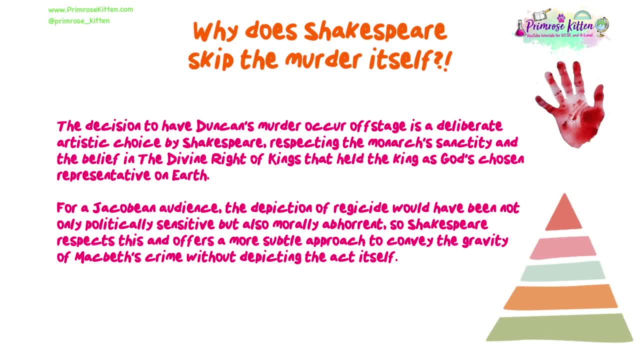 then either It's because it happens off-stage Now. the decision to have Duncan's murder occur off-stage is a deliberate artistic choice by Shakespeare. It respects the monarch's sanctity and the belief in the divine right of kings that held the king as God's chosen representative on. 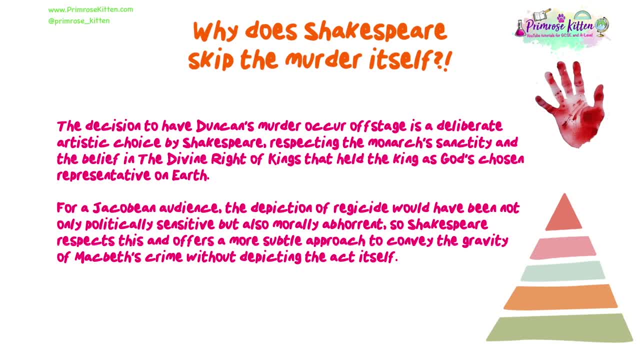 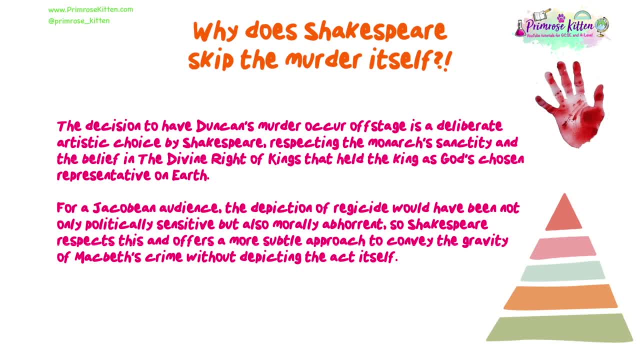 gravity of Macbeth's crime without depicting the act itself. Don't forget: this play isn't about the murder. it's about the consequences of people who try to commit regicide or do commit regicide. so that's what it's all about. It shouldn't be a focus of kind of glamorising murder. 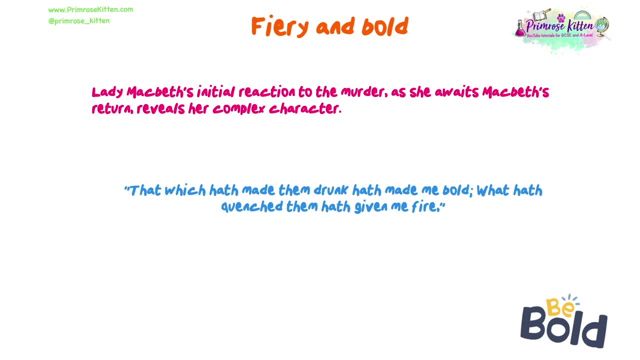 Now, at the start of the scene, Lady Macbeth's, kind of on her own. She's awaiting Macbeth's death, and it's actually been done, and it actually does reveal her complex character. She says that which hath made them drunk, hath made me bold, what hath quenched them, hath given. 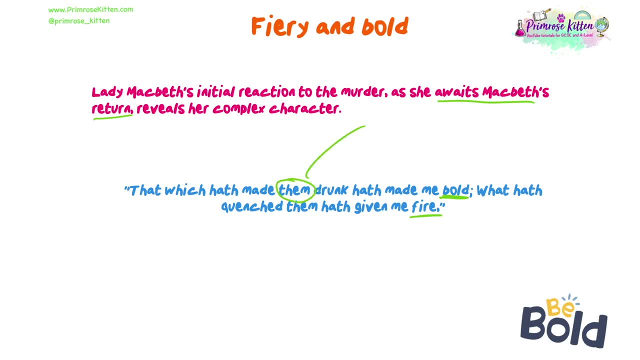 me fire. Now, when she mentions them, she's just talking about the two gods, but they all go into frame And what she's saying is she's kind of contrasting the effects of alcohol on the gods with the courage it's instilled in her While they're being framed. it's allowed her to proceed. 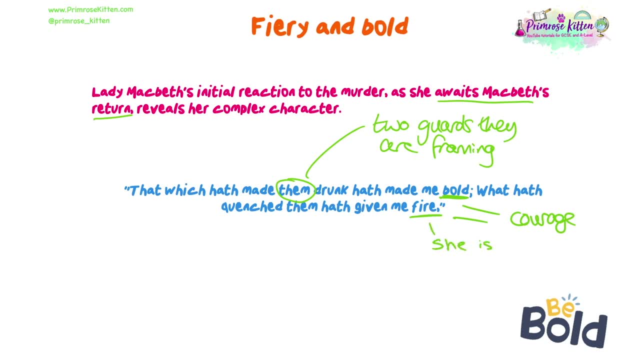 with her plans. So the use of the word frame, the use of the word murder is a way of saying the use of bold and fire emphasises her determination and her fiery spirit, And those are characteristics that propel her actions earlier in the play. Obviously, fire connotes. 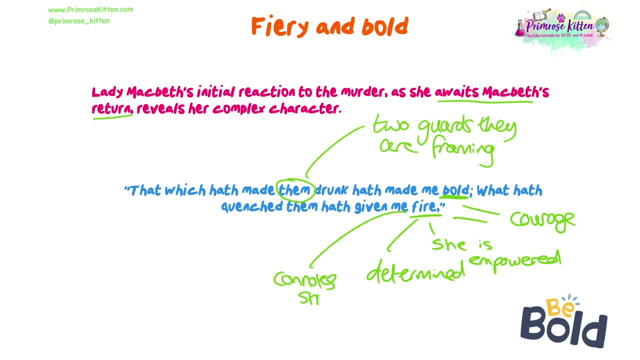 strength and even destruction, but her tone almost conveys pride in this. She's proud that she is bold and fiery. She seems almost empowered by the fact that they will remain undetected because of the framing of the gods. However, in the same conversation, in the same piece of dialogue, her 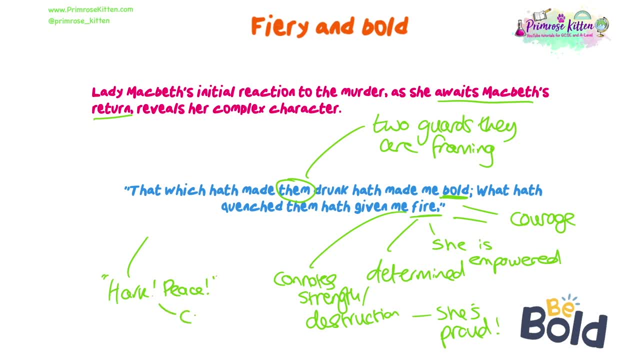 voice seems to be more powerful than ever before. She seems to be more confident than ever before. She seems to be more confident than ever before. She seems to be more confident than ever before. It was that owl that shrieked. betrays a flicker of vulnerability. 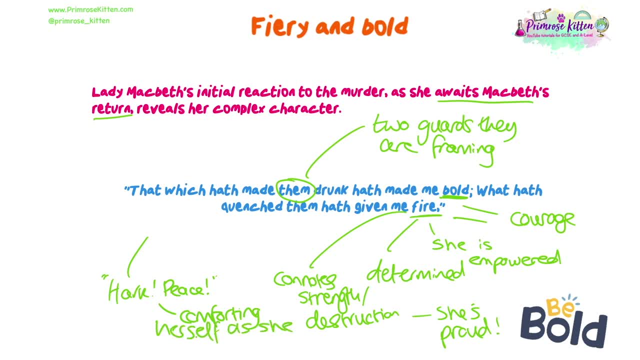 hinting at the internal conflict and fear that underpin, potentially, her facade of strength. She appears frightened by every sound, in fear that the plan will be uncovered should any single guest wake up. Now, don't forget, she's the powerful one in terms of. 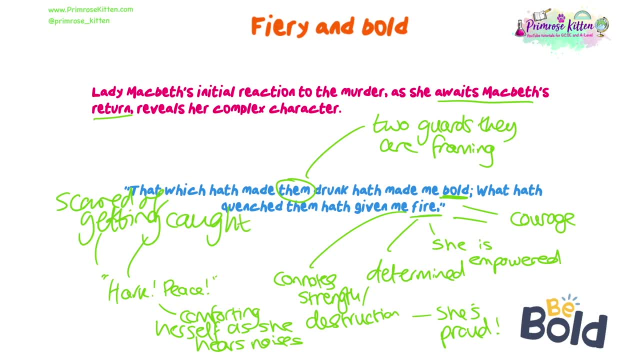 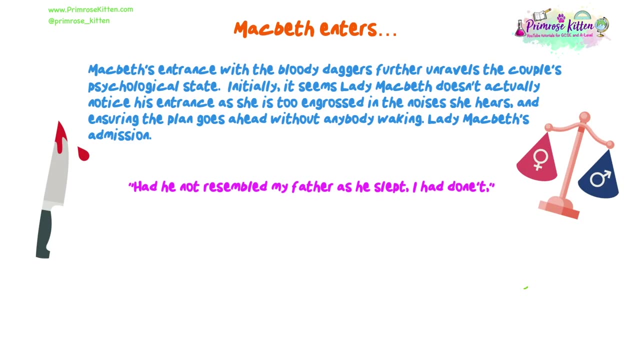 the dynamics in the relationship at the moment. but there are subtle hints early on that potentially she's not as strong as she sort of portrays herself to be And that does track. considering later on in the play we obviously see her mental sort of downfall. Macbeth's entrance with the bloody daggers. 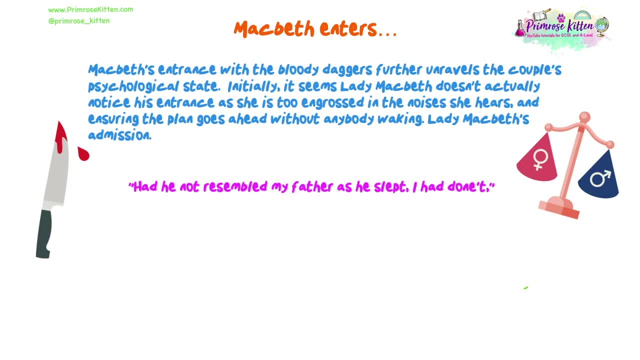 further unravels the couple's psychological state. Initially, Lady Macbeth doesn't actually notice his entrance because she's still too engrossed in the noises that she can hear and thinking about the plan going ahead successfully without anybody waking. She says to herself: had he not resembled. 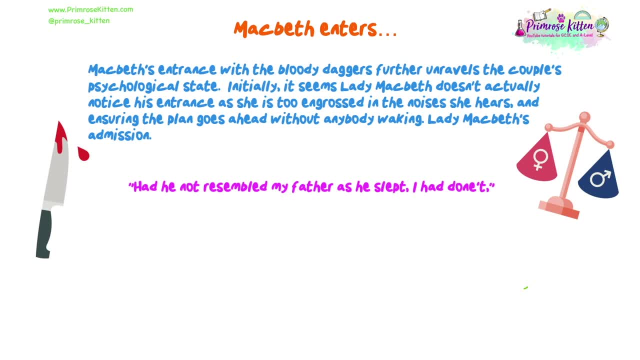 my father as he slept, I had done it, Which essentially means that if King Duncan didn't look like her father, then she would have done it herself. And this reveals quite a few things. Firstly, it reveals a moral boundary that she is unwilling to cross. It's a moment of weakness. 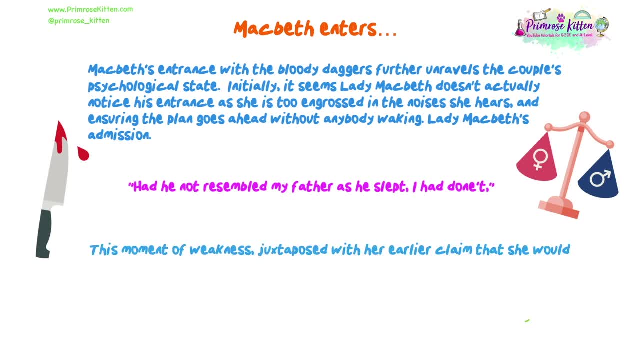 and juxtaposed with her earlier claim that she would dash out the brains of her own child, actually introduces a complex interplay between maternal instincts and reverence to her father and a sense of self-doubt. It suggests that her capacity for violence is lessened somewhat by 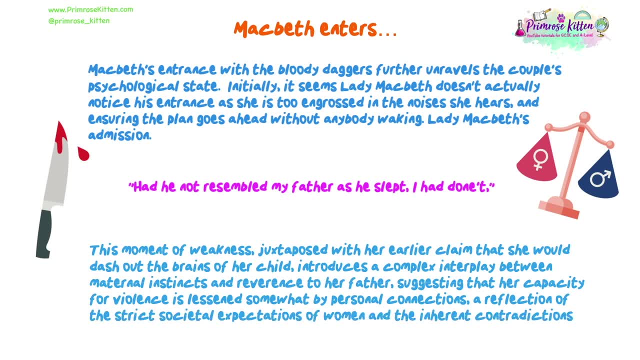 personal connections. It's a reflection of strict societal expectations of women, because as a woman, you were supposed to see your husband, and originally your father, as essentially the two most important people in your life, or the two most important men in your life: First your father, then your husband. It also shows real inherent contradictions within her. 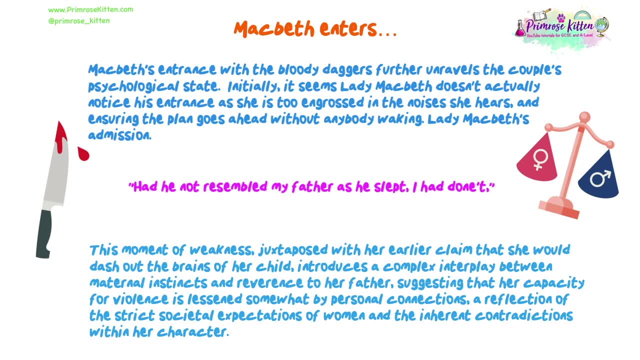 character, and I just mean there that a lot of things that she says kind of go in the way of her character. So she's not the kind of person that would go against previous things that she says and that might explain later why we see her suffering the way that she does. 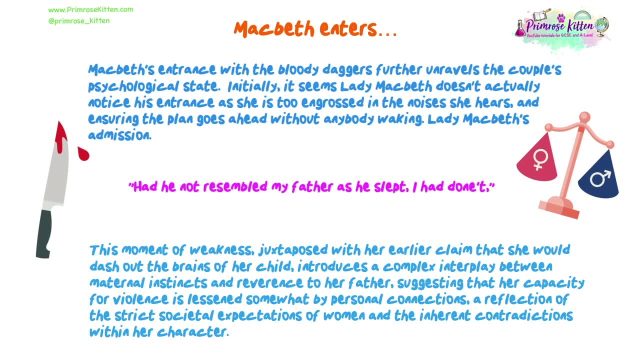 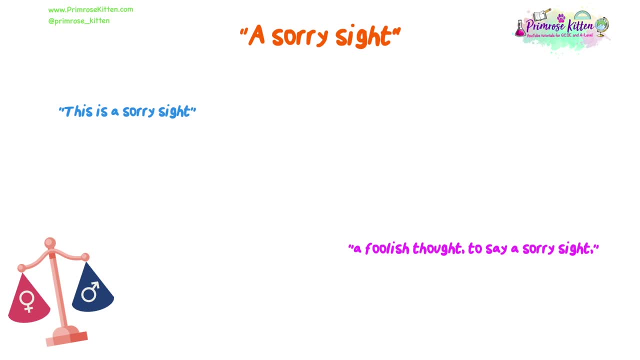 because she's so complex and there's a lot of things. there's a lot of conflict inside her In their exchange. when Macbeth has returned- and Lady Macbeth is aware of this- it's fraught with panic and urgency. Macbeth's immediate regret when he says this is a sorry sight. 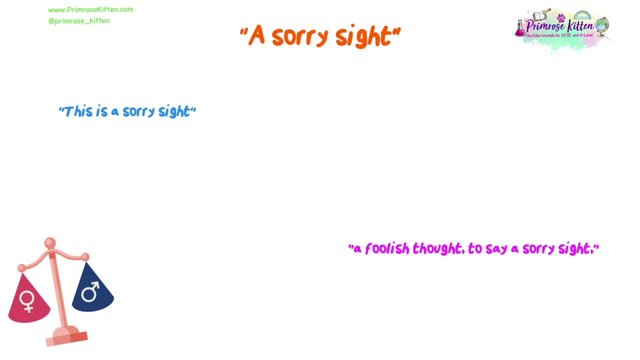 and Lady Macbeth's immediate regret when he says this is a foolish thought, to say a sorry sight, and it showcases her attempt to maintain control and suppress any acknowledgement of guilt. This dynamic, this relationship, again reveals a power imbalance where Lady Macbeth assumes a 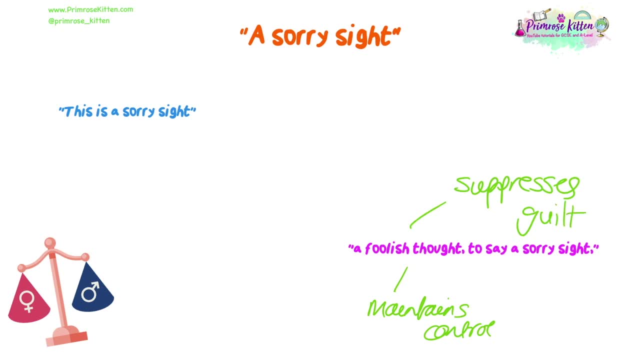 dominant role, striving to bolster Macbeth's resolve despite her own subtle fears. One thing I would say here, though, is that where Macbeth's fears arise from a place of regret and fear of his own damnation, Lady Macbeth's fears at present are mostly regarded as a 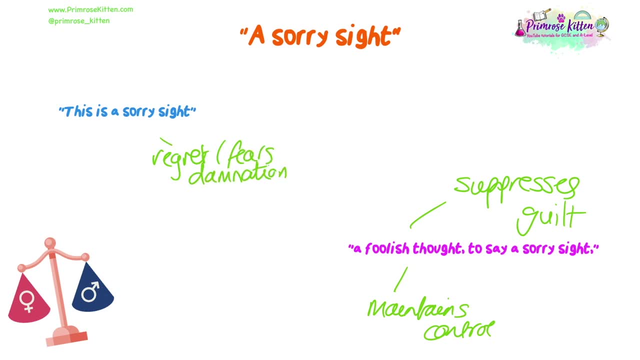 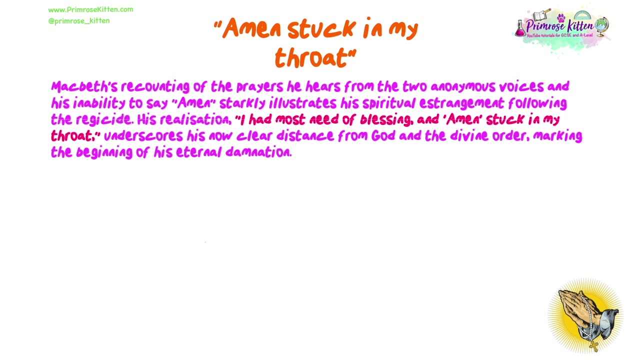 getting caught and are clearly not enough to change her perceptions after the event has taken place. Macbeth's recounting of the prayers he hears from the two anonymous voices and his inability to say Amen starkly shows his spiritual estrangement following the regicide. 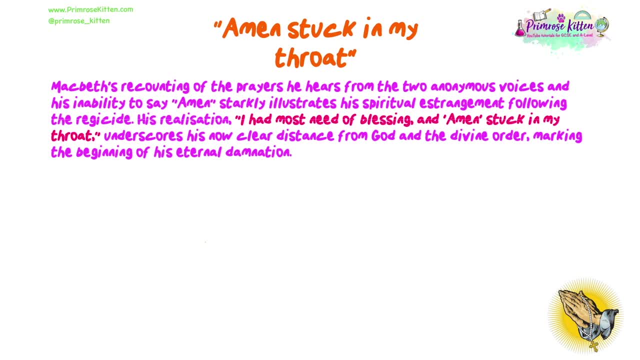 and when I say estrangement I just mean his separation from his spirituality. His realisation I had most need of blessing than Amen stuck in my throat underscores his now clear distance from God and the divine order marking the beginning of his eternal damnation. It's quite a visceral image. 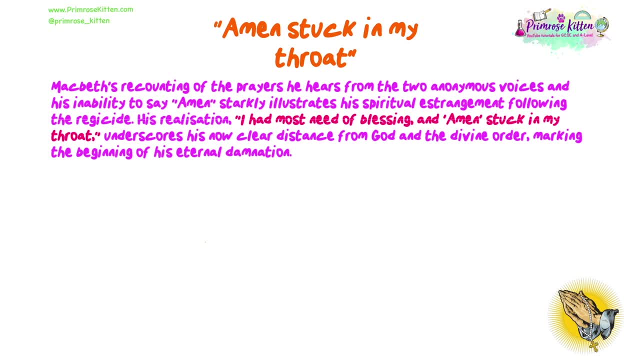 and by visceral I mean you can almost feel it yourself. it's painful and it conjures images of coughing or choking, reflecting the pain he feels without his ability to seek God. This moment, reflective of the biblical principle that sin separates man from God. 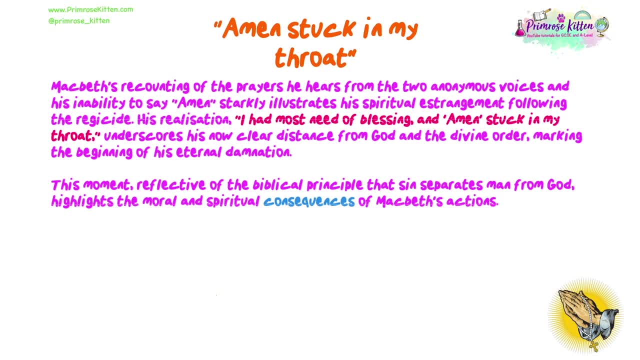 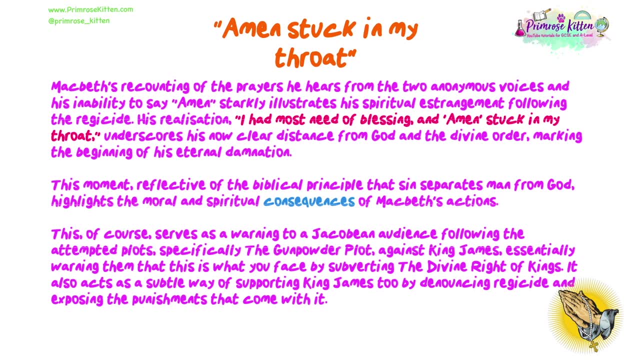 highlights the profound moral and spiritual consequences of Macbeth's actions. This, of course, serves as a warning to a Jacobean audience following the attempted plot- specifically the gunpowder plot- against King James, essentially warning them that this is what you face by subverting the divine right of kings. It also acts as a subtle way of supporting King. 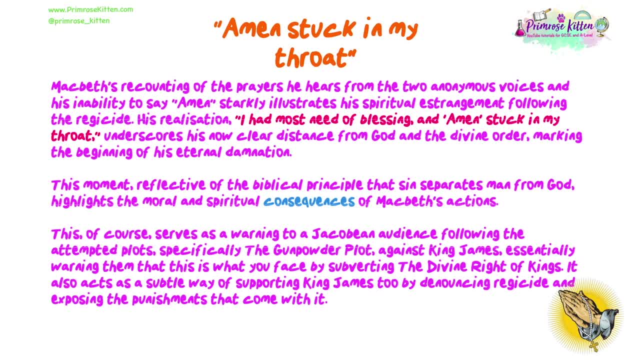 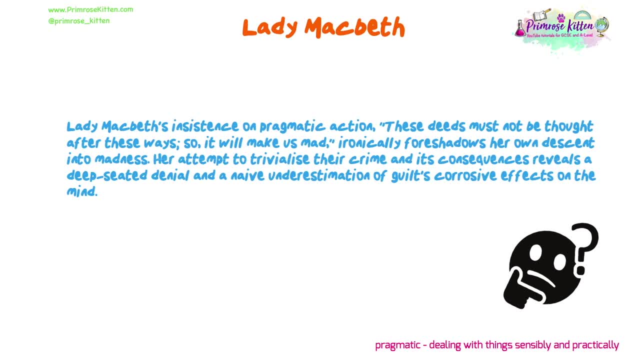 James too, by denouncing, or in other words criticising regicide and exposing the punishments that come with it. Now Lady Macbeth insists that they get moving so they don't get caught, and her insistence on pragmatic action where she says these deeds must not be thought after these. 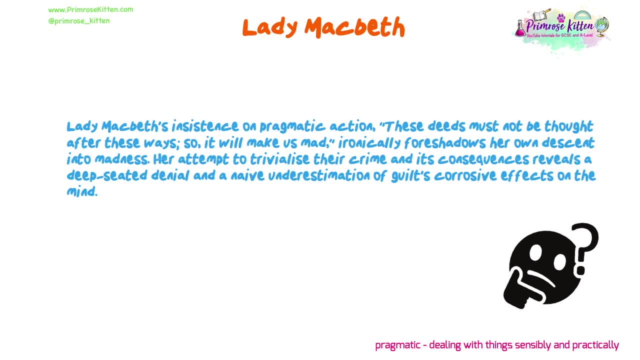 ways, so it will make us mad, is ironic because it foreshadows her own descent into madness, when she obviously ends up thinking about it too much. Her attempt to trivialise their crime and its consequences reveals a deep-seated denial and naive underestimation of guilt's corrosive effect. 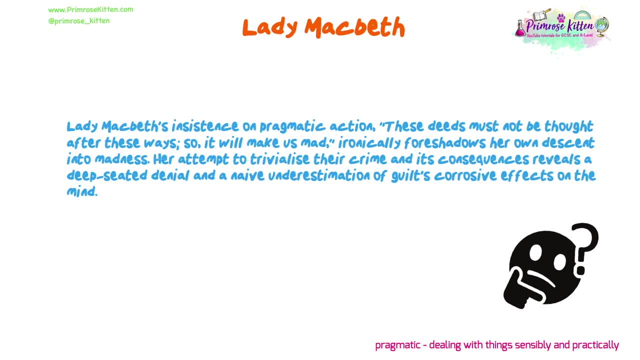 She is an old woman who has tried to make her life seem like nothing and make it seem like it's silly, is kind of underestimating just how painful it's going to be and how much suffering it's going to cause her internally. 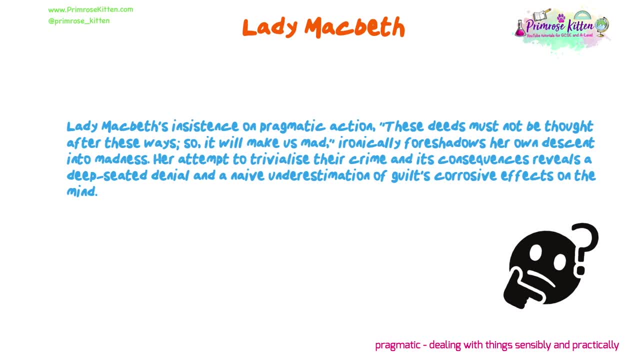 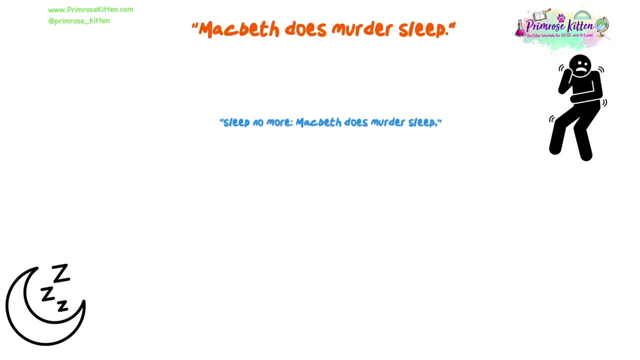 And you almost start to see her lose her patience more and more from here. she knows they need to be quick to avoid being caught. Macbeth's hallucinations of a voice declaring sleep no more. Macbeth does murder. sleep metaphorically links that act of. 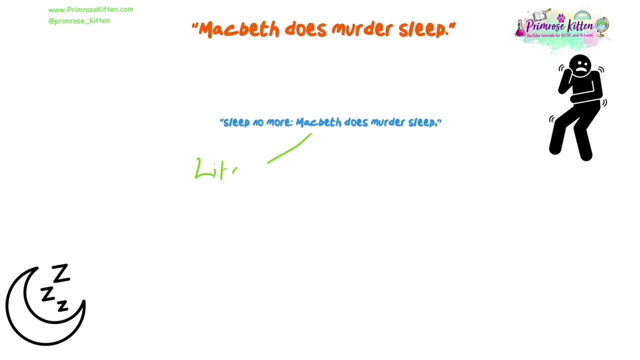 of regicide to the disruption of natural and moral order. Literally, Macbeth has murdered someone sleeping, but metaphorically, when we think of the connotations of sleep being at peace, he has murdered peace and therefore disrupted what was natural and orderly about the world. Not only has 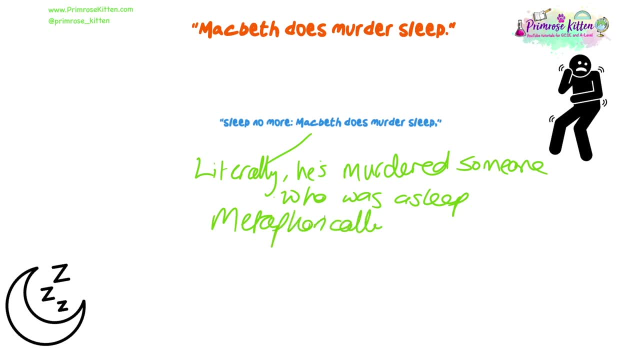 this caused turmoil within Macbeth's soul, but because he has disrupted the great chain of being what Jacobians believed was a natural and god-given hierarchy, there is now turmoil in Scotland too, So that repetition of sleep no more as well throughout the conversation that follows by. 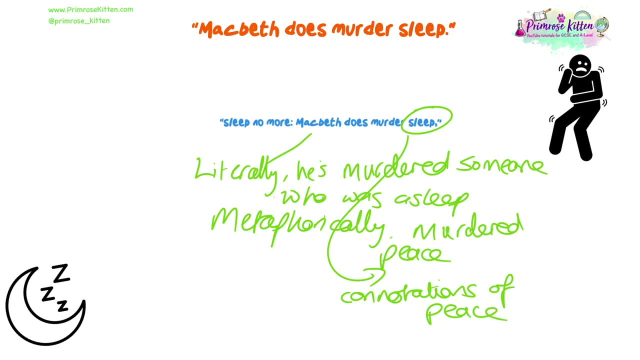 both the voice and Macbeth, further magnifies the loss of peace and innocence he will experience from here on out. Now I just want to be clear here. the great chain of being was an order set out for all living things in the world, and actually even non-living things too. So there's a hierarchy. 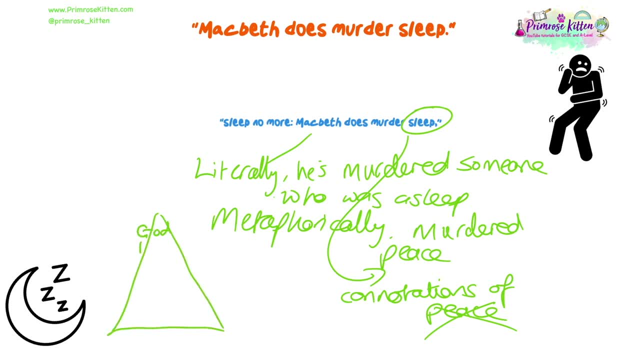 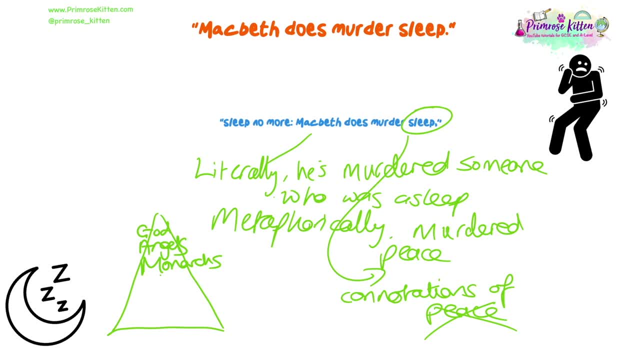 Then common sort of normal people, animals, plants, even non-living things. So because Macbeth has disrupted that right sort of in the middle of that chain of kings or queens, taking those out, it's disrupted what would have been seen as a really natural order or a natural 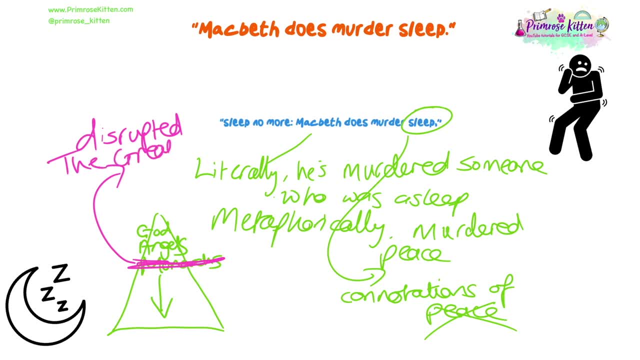 hierarchy. So that's why there's going to be turmoil not only within himself, but within Scotland as well. Now there's an interesting link that you can make here, and it's back to Act 1, Scene 3, where the witches give him his predictions. They say first: all hail Macbeth, hail to the Thine of Glamis. 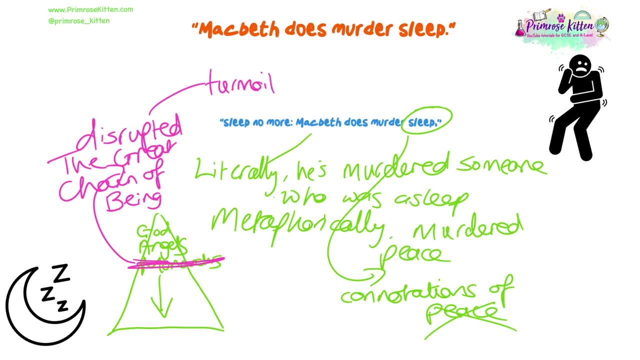 which is what he is when he first meets them. Then all hail Macbeth. hail to the Thine of Cawdor, which is what he will next become. Happens immediately after the witches have gone, actually. And then, third, they say: all hail Macbeth, that shall be king hereafter. Now, in this scene, 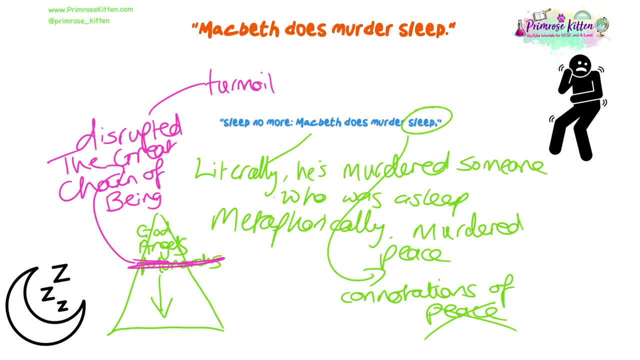 Act 2, Scene 2,. he hears the voice specifically say: alarms hath murdered sleep, and so he's believes and he says this: therefore: Cawdor shall sleep no more, Macbeth shall sleep no more. So when he hears the voice saying that Glamis hath murdered sleep, he interprets that as Cawdor shall. 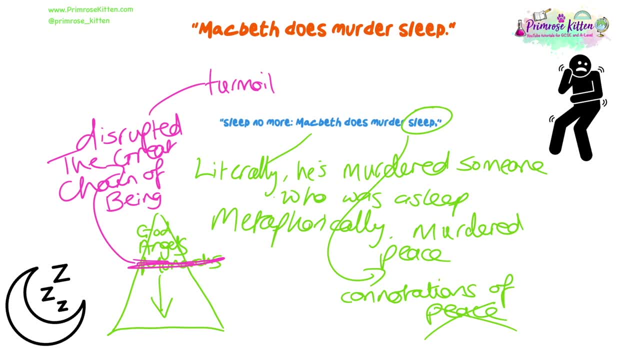 sleep no more. Macbeth will sleep no more. He's concerned he will never be able to sleep peacefully again because of what he's done. Now if you link that back to those witches' predictions, the witches' prophecy kind of ominously echoes through his mind. It's in his head. 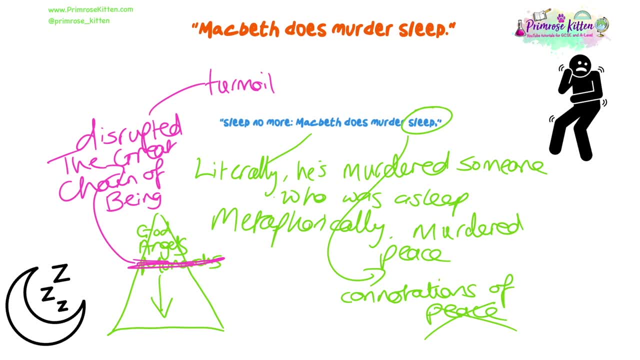 obviously he wants to be king, But notice that he mentions nothing of becoming king. He says: Cawdor shall sleep no more, Macbeth shall sleep no more. He says nothing about being king. He doesn't say anything like the king shall sleep no more. He mentions nothing of a king like they did. He only mentions Glamis. 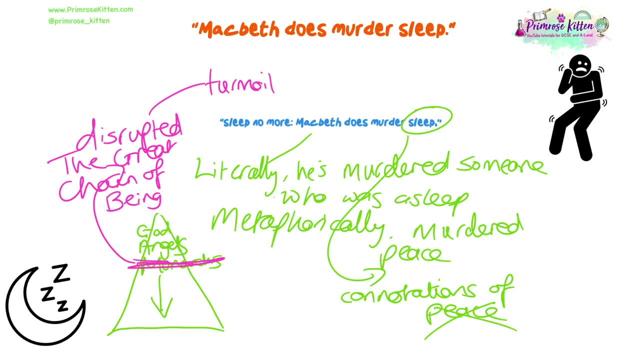 and Cawdor, which suggests that deep down, perhaps even subconsciously, he knows, even if he does get the crown, he will never truly be a real king, because of course he is not going to be chosen by God. And this theory does seem to make sense because later on you only have to look at how paranoid he. 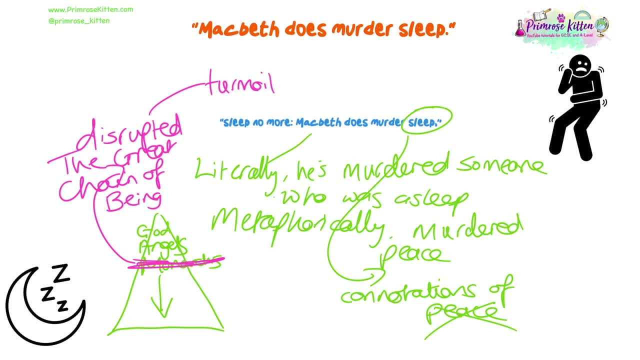 gets at the thought of anybody getting in his way. He knows that he's not supposed to be rightfully there. He's not a rightful king like Duncan was or like Malcolm should be. He defends his title obsessively, perhaps because deep down he knows it's not really his to hold. Now, if you can spot. 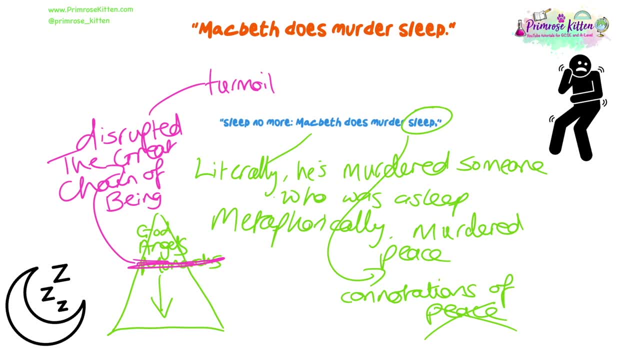 those clever little links and explain how moments in the scene you're talking about can link back to previous ones or can force you back to the previous ones, you'll be able to find a way to shadow future ones. It's a really, really brilliant skill to have in your essays. 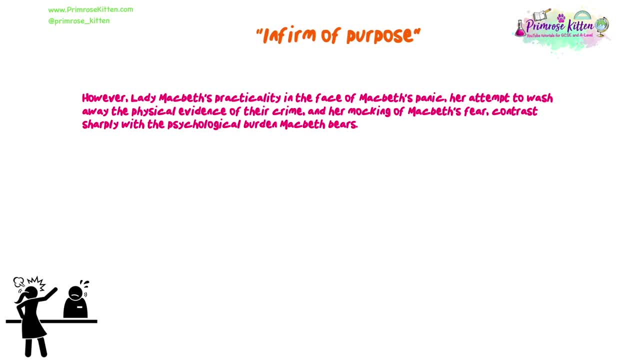 Now this is really where Lady Macbeth starts to lose her patience, because he is still absolutely freaking out with what he can hear and she just wants to be practical. She wants to make sure they don't get caught. She's become really urgent and impatient now. So Lady Macbeth's practicality in 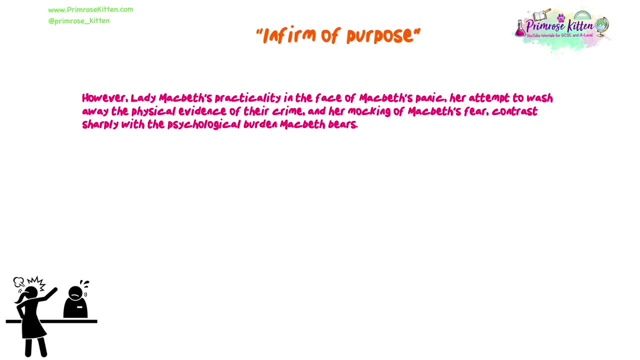 the face of Macbeth's panic, her attempt to wash away the physical evidence of their crime and her mocking of Macbeth's fear contrasts really short. So Lady Macbeth's practicality in the face of Macbeth's panic, her attempt to wash away the physical evidence of their crime and her mocking of Macbeth's fear contrasts really short. Lady Macbeth's practicality in the face of Macbeth's panic, her attempt to wash away the physical evidence of their crime and her mocking of Macbeth's fear contrasts really short. Lady Macbeth's practicality in the face of Macbeth's panic, her attempt to wash away the physical evidence of their crime and her mocking of Macbeth's fear contrasts really short. 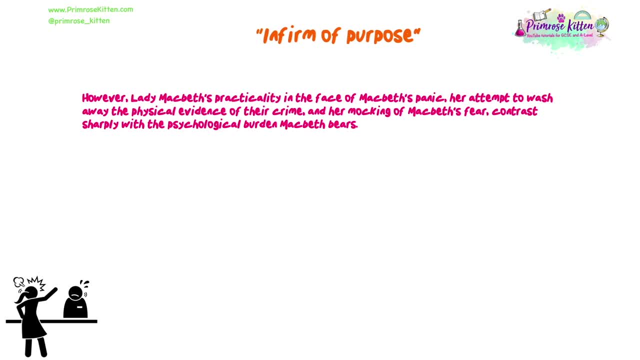 Lady Macbeth's practicality in the face of Macbeth's panic, her attempt to wash away the physical evidence of their crime and her mocking of Macbeth's fear contrasts really short. Lady Macbeth's practicality in the face of Macbeth's panic, her attempt to wash away the physical evidence of their crime and her mocking of Macbeth's fear contrasts really short. 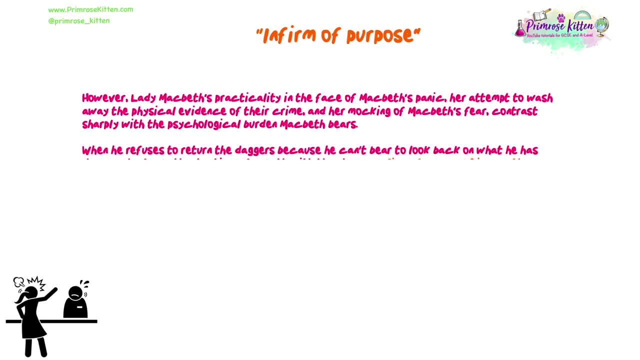 Lady Macbeth's practicality in the face of Macbeth's panic, her attempt to wash away the physical evidence of their crime and her mocking of Macbeth's fear contrasts really short When he refuses to return the daggers because he can't bear to look back on what he has done. 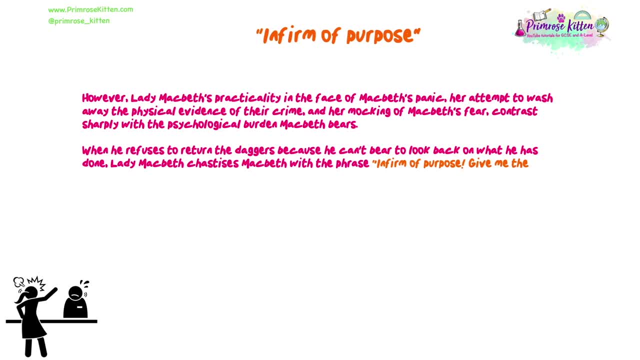 Lady Macbeth chastises Macbeth with the phrase infirm of purpose, give me the daggers. This critical moment illuminates her frustration with Macbeth's faltering mental state. The term infirm, meaning useless in this sense, suggests weakness or a lack of strength, indicating Lady. 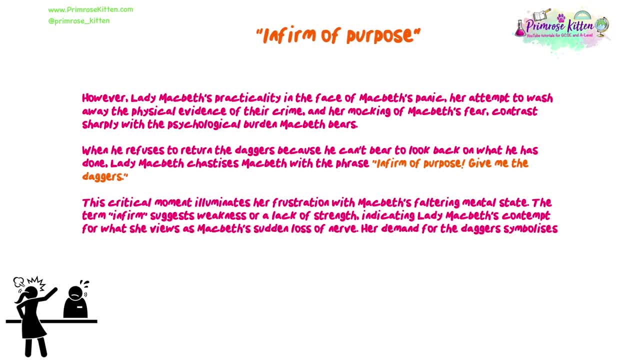 Macbeth's contempt, or anger or frustration, or even hatred for what she views as Macbeth's sudden loss of nerve. Her demand for the daggers symbolises her willingness to take control of the situation. She's asserting herself as the more decisive of the two in the face of their deed. 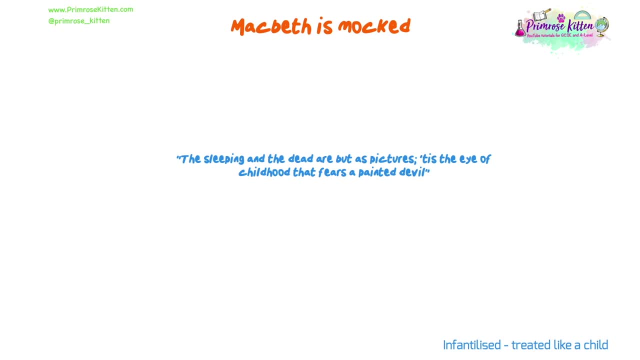 In this same conversation and moment she says the sleeping and the dead are, but as pictures. It is the eye of childhood that fears the painted devil, and this further reinforces her attempt to minimise the gravity of their actions and to steer Macbeth, maybe even herself, against remorse and 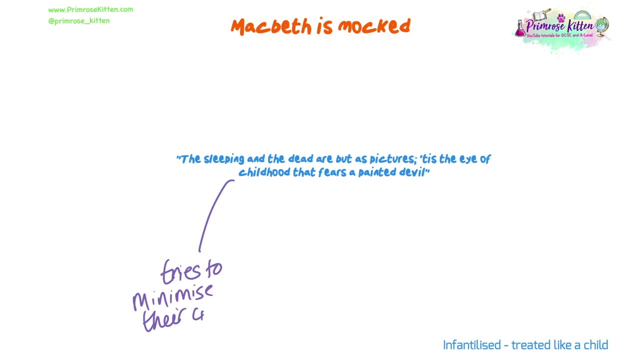 fear. By comparing the sleeping and the dead to mere images or paintings, she suggests that the dead, like the sleeping, are actually no threat at all. They are static, they can't move, they're harmless, and she likens that to the inanimate subjects of paintings. By using this analogy or this: 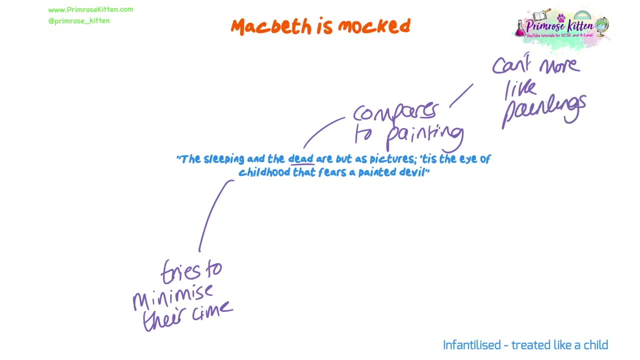 comparison, Shakespeare shows her naive attempt to distance themselves from the guilt of the murder by dehumanising their victim, reducing Duncan to nothing more than just a dead body who has no life, No power to affect the living. If he is dead, he can't cause them any more. suffering is essentially 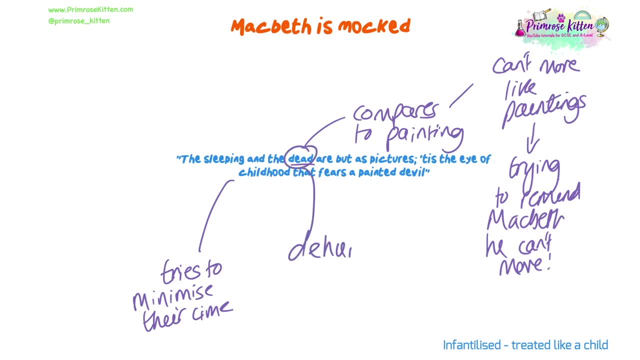 what she's arguing, which is very naive of her, as we know. The reference specifically to that eye of childhood that fears the painted devil is particularly interesting because she suggests that his fears are irrational and childish. Lady Macbeth's use of this imagery is an attempt to 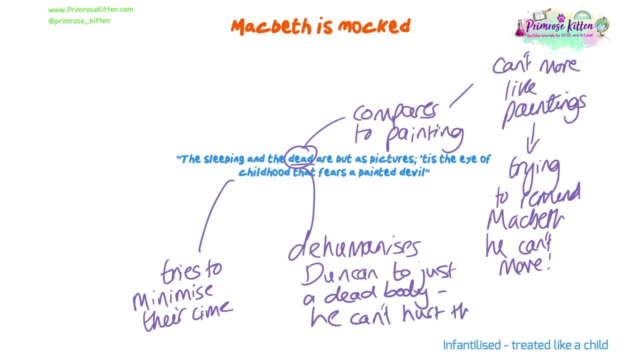 shame Macbeth for his cowardice, likening his fear to that of a child scared of fictional monsters. almost We might link this to the theme of the book, which is the idea of a child scared of the game of appearance versus reality, since she did just admit that she would have done it herself. 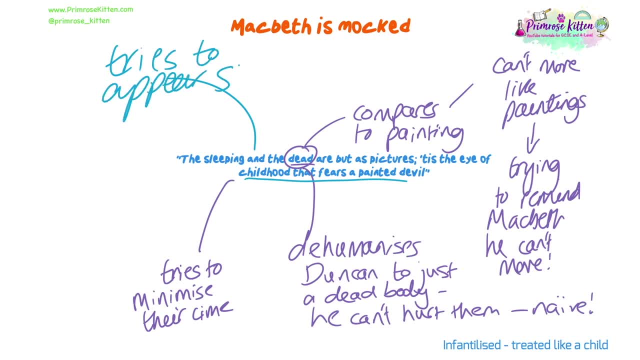 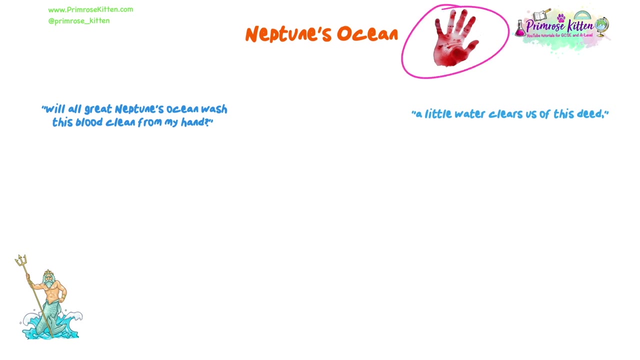 if King Duncan didn't look like her father. So it suggests she even has to put on a front before her own husband too. It therefore reflects Lady Macbeth's desperation to maintain their façade of normalcy and control. The motif of hands symbolising action and guilt becomes a recurring. 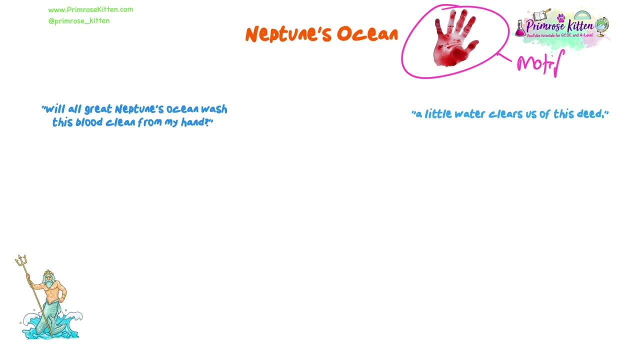 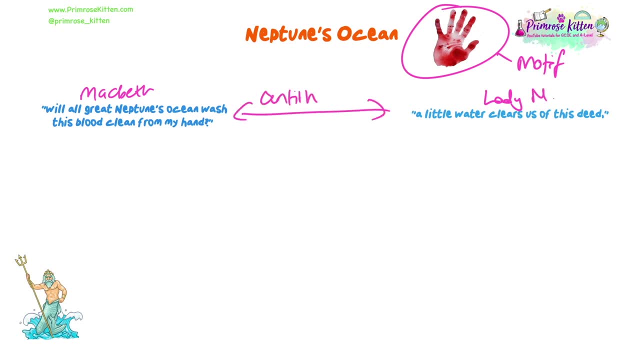 or opposite, in other words, perceptions of guilt. While Lady Macbeth underestimates the stain of their crime, Macbeth recognises its damaging impact. It foreshadows their inescapable and tragic downfall. Now I do think it's worth looking really closely at this quotation from 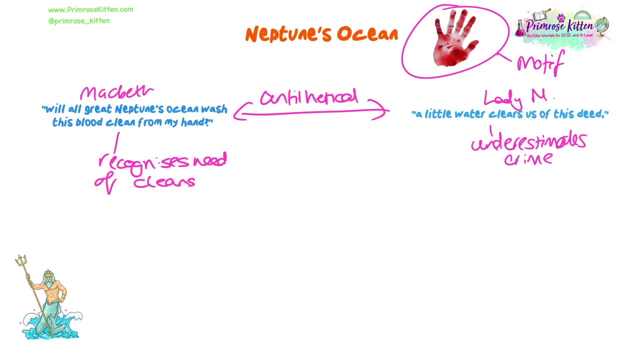 Macbeth because he recognises God's rejection As, don't forget, they believed the monarch was chosen by God. By calling on Neptune, the Roman god of the sea, Macbeth acknowledges his transgression against God and naively looks elsewhere for cleansing and redemption. His plea also reflects a sense of desperation and 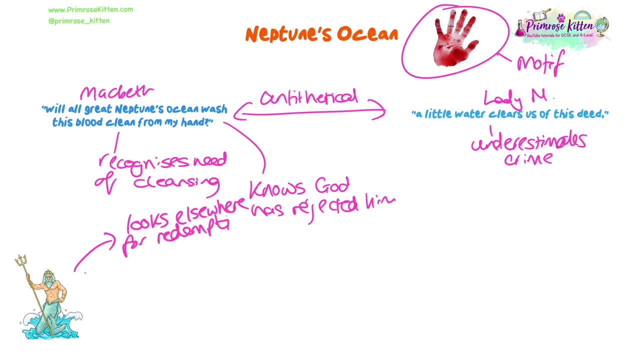 resignation as he realises the enormity of his crime and the inevitable consequences that await him. He knows he can't turn to his own god anymore. so he looks elsewhere, showing his acceptance of damnation. Now in the Bible, if you want to kind of link here in terms of context, it says you shall not have any. 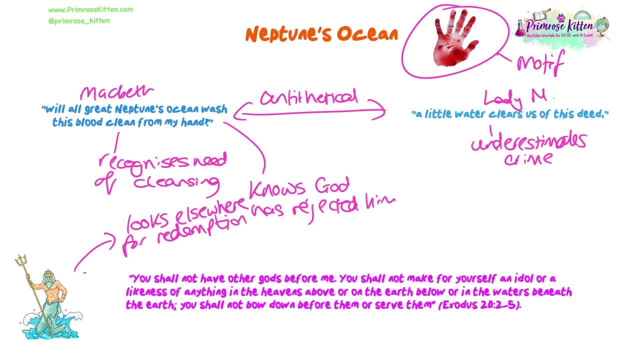 other gods before me. You shall not make for yourself an idol or a likeness of anything in the heavens above or on the earth below or in the waters beneath the earth. You shall not bow down before them or serve them. Now, essentially, what that means is that in the Bible it argues there: 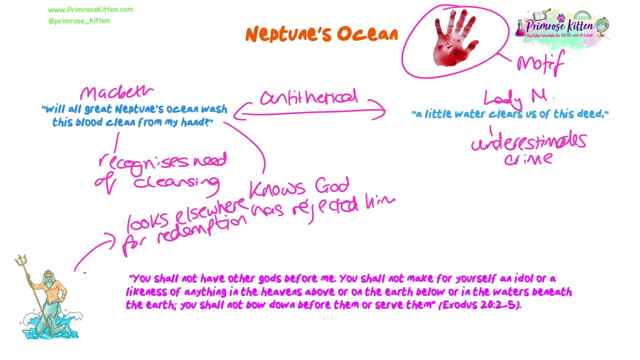 should be no other god for you to worship before God himself. Now, ironically, Macbeth seeks help elsewhere, but by seeking another omnipotent force away from the Christian god that he worships, he commits further sin, as in the Bible, Obviously, as we've. 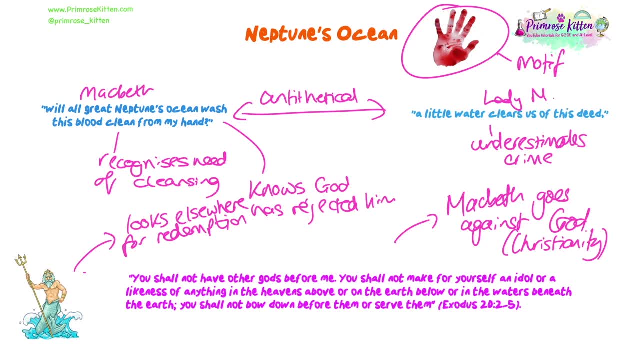 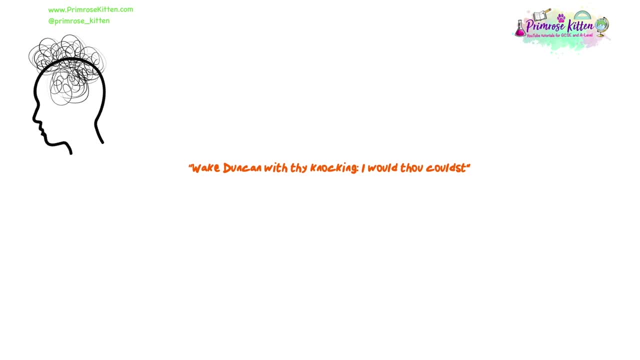 just seen there. it literally warns against putting another god before him. Now, finally, towards the end of the scene, they try to compose themselves and initiate their facade of innocence. They get their nightgowns on and look as if they've been awoken themselves, That's. 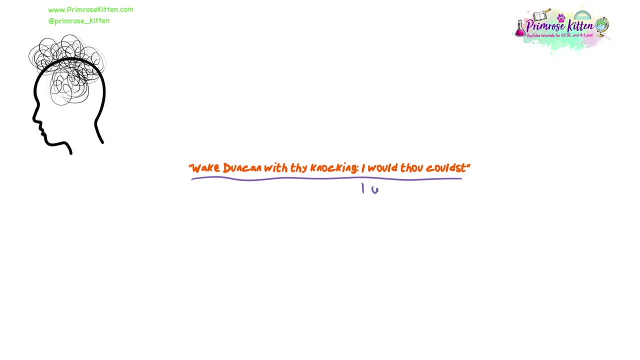 the intention. That's what Lady Macbeth says. The final line of the scene is almost sombre and poignant. It's quite a quiet and sombre moment for Macbeth and the regret is almost palpable. We can almost feel it. Macbeth says: 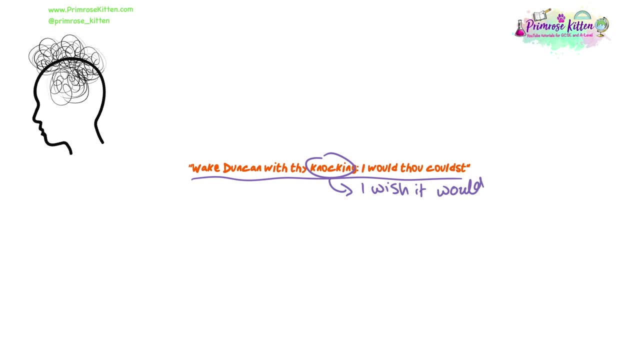 And all that means is I wish that the knocking that I can hear would wake Duncan up. And in wishing to awaken Duncan with the knocking, Macbeth expresses a futile, or pointless, in other words, regret, Desire for redemption. He knows it's futile, He's desperate to escape his sin And it's a clear 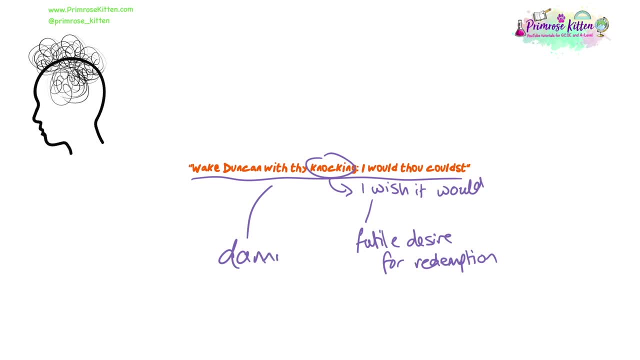 acknowledgement of his remorse and the fact that his sin is definitely irreversible. This sombre conclusion to this scene emphasises the enormity of Macbeth's crime and the play's central themes of ambition, moral corruption and the quest for power at the soul's expense. 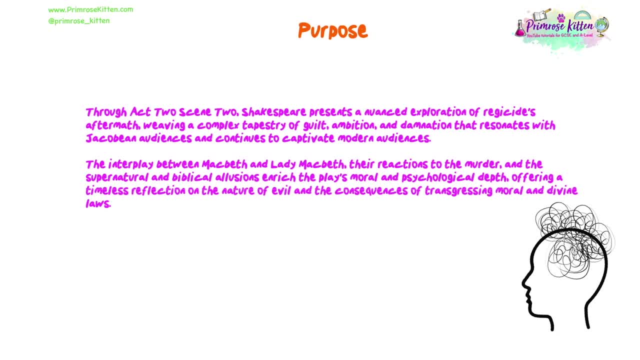 Now in terms of the purpose, in Act 2, scene 2, we get this really deep exploration of Regicide's aftermath. We look at themes of guilt, ambition and damnation and how it resonates with a Jacobean audience and continues to captivate. 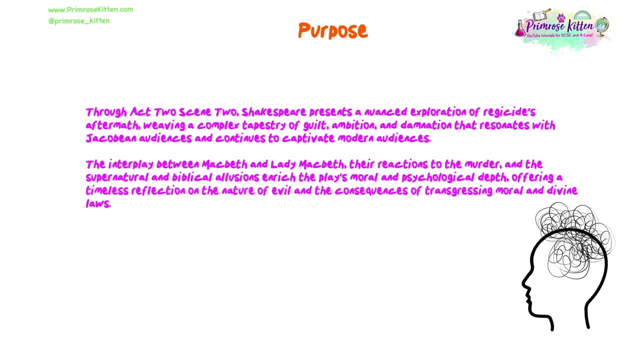 modern audiences too. The interplay between Macbeth and Lady Macbeth, their reactions to the murder and the supernatural and biblical allusions enrich the play's moral and psychological depth. It offers a timeless reflection on the nature of evil and the consequences of transgressing. 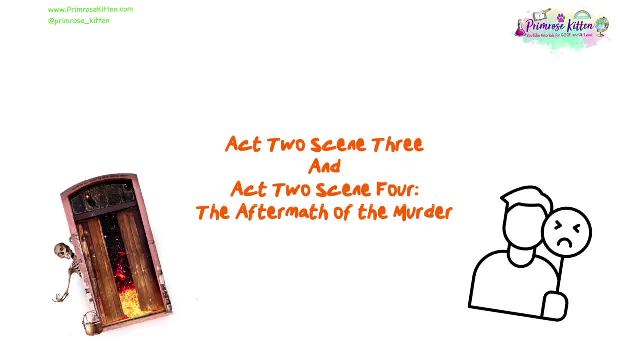 moral and divine. In Act 2, scene 3 of Shakespeare's Macbeth, the introduction of the Porter scene serves as a momentary relief from the play's escalating tension and horror following the sinful act of Regicide committed by Macbeth. Now, this is a scene you don't want to ignore, and it actually 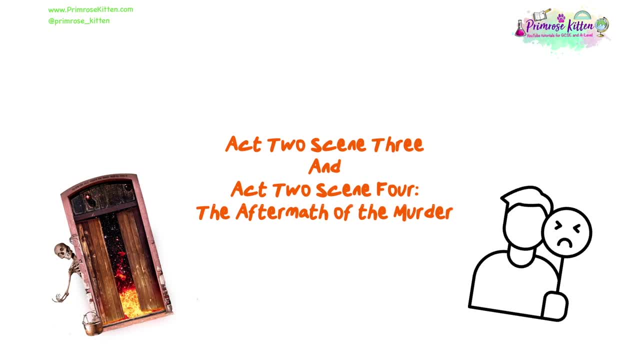 came up in another exam one year and it gets glossed over often because of time constraints at school. Now it serves as an important reminder to know the whole text. That doesn't mean you need to memorise everything, but it does serve as an important reminder to know the whole text. 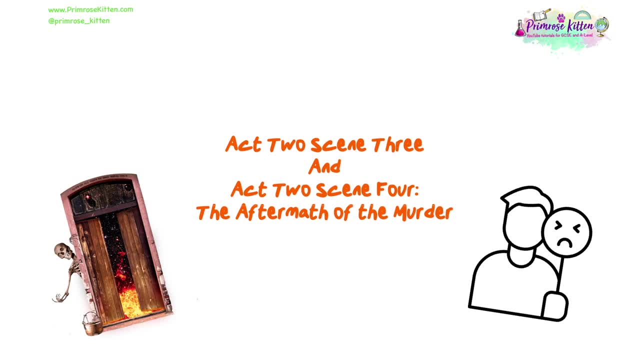 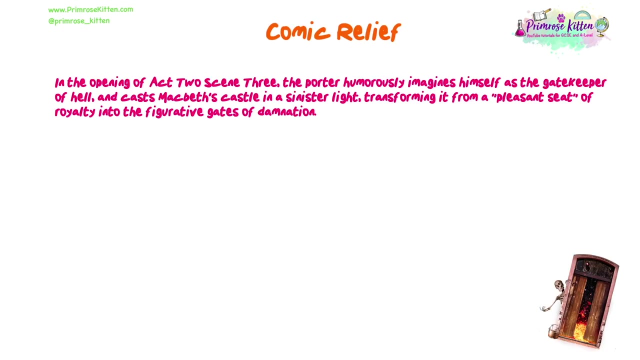 So I've sort of combined scene 3 and scene 4 for this video, purely because I wanted to explore generally the immediate aftermath of the murder. Now, essentially at the start, the Porter humorously imagines himself as the gatekeeper of hell and he casts Macbeth's castle in a really sinister light, transforming it from. 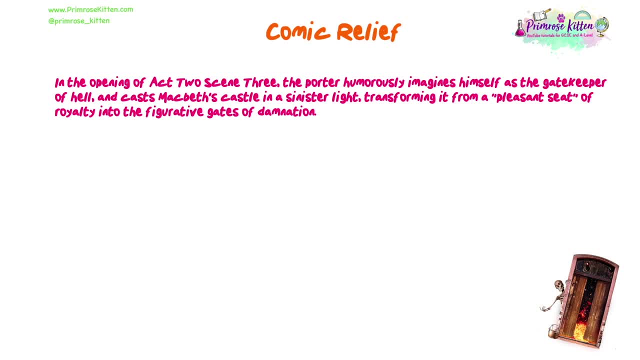 a pleasant seat of royalty into the figurative gates of damnation. By this I'm just referring to the fact that the castle was initially described by Duncan for its welcoming atmosphere, but it has become the scene of the king's murder, effectively sentencing Macbeth to eternal damnation. 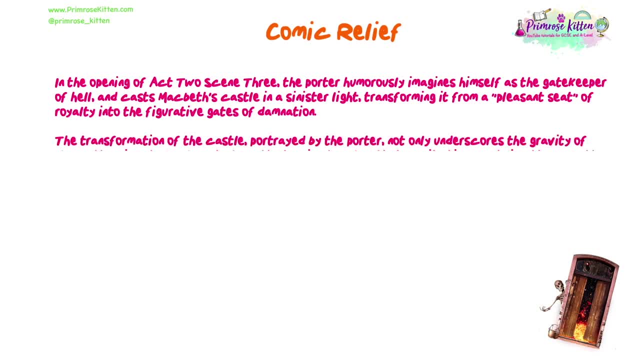 The transformation of the castle portrayed by the Porter not only underscores the gravity of Macbeth's sin, but also foreshadows the tragic downfall that awaits him, much like the souls the Porter jestingly admits to hell. The comparison of Macbeth to Lucifer later in the play cements. 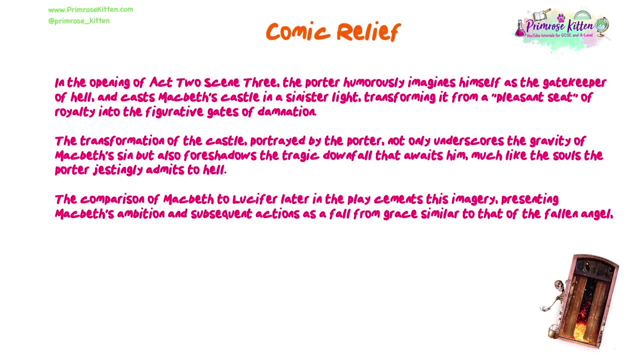 that are seen in the play. The Porter's role is defined in Macbeth's ambition and subsequent actions as a fall from grace akin to that of the fallen angel. Through the Porter's drunken ramblings, Shakespeare subtly alludes to the castle's newfound status as a gateway to hell, a place where deeds 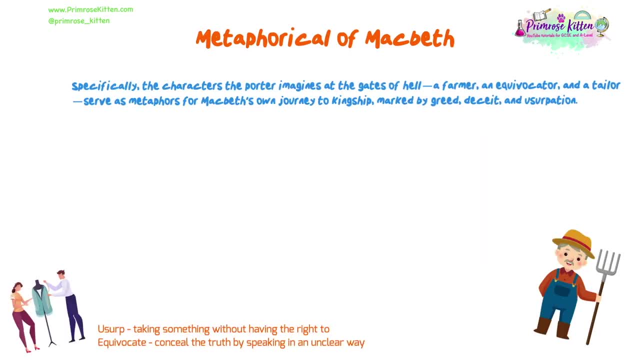 of greed, deception and treachery lead to one's ultimate ruin. Now, specifically, the characters the Porter imagines at the gates of hell are a farmer, an equivocator and a tailor. They serve as metaphors for Macbeth's own journey to hell. 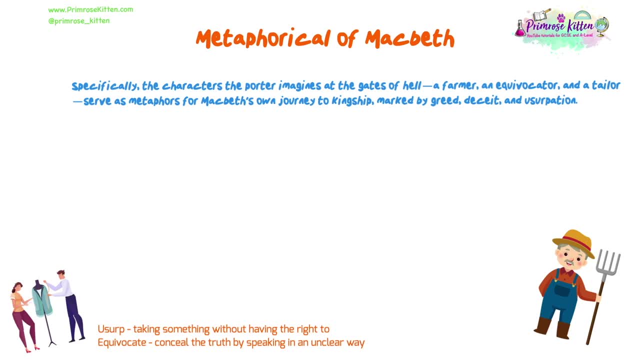 journey to kingship marked by greed, deceit and usurpation. First, a farmer who arrives at the gates because of his own greed mirrors Macbeth's ambition and the dire consequences it brings, foreshadowing his inevitable punishment. So just for this next one, an equivocator is a person who 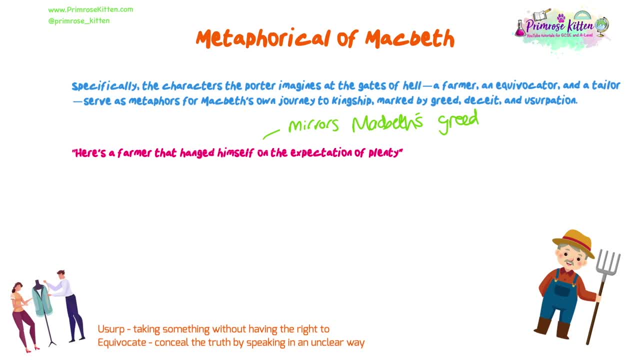 carefully words things and speaks in a really unclear way, deliberately to conceal the truth. So where it says, here's an equivocator that could swear in both the scales, against either scale, who committed treason enough for God's sake, yet could not equivocate. to heaven, reflects Macbeth's. 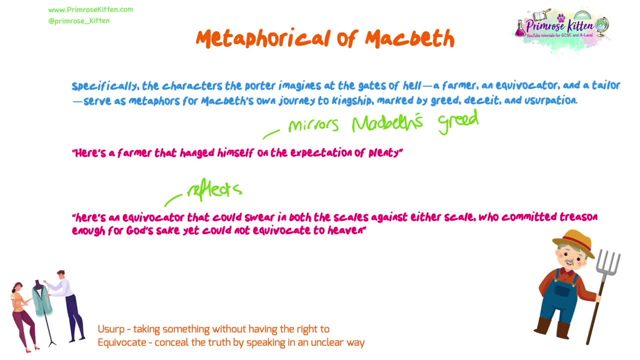 moral ambiguity and his manipulation of the truth to achieve what he wants, And obviously we're going to see a lot of that in the scenes that follow. The porter implies that this equivocator he's imagining could argue for both sides with his clever wording, And this one's a really interesting. 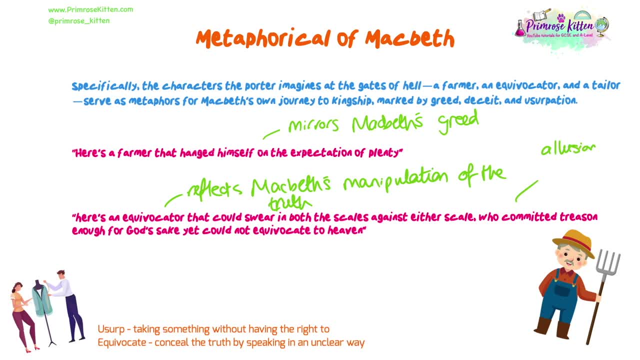 one, actually, because Shakespeare's reference to the equivocator holds kind of a particular resonance for the audience at the time- Contemporary audience- as it draws a kind of parallel to Father Garnet, who was involved in the Gunpowder Plot slightly. Now he was a priest arrested for his complicity in the 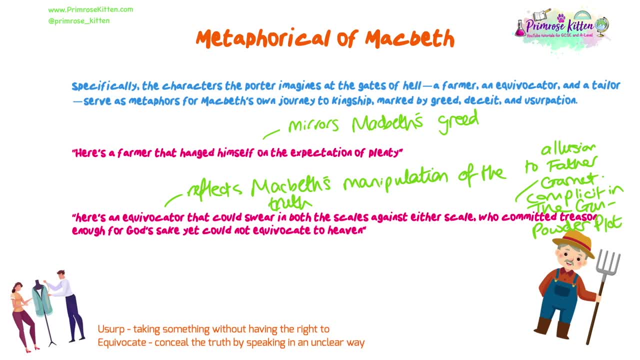 Gunpowder Plot because he famously used equivocation to avoid being executed. He was criticised for his equivocation when hiding the truth about a confession he heard from one of the plotters. So he wasn't directly involved, but he was complicit. So there, mockery, and 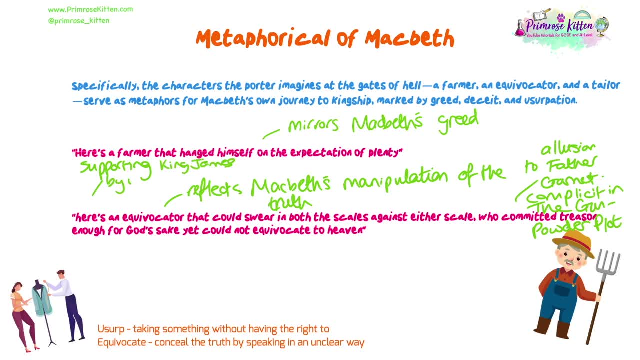 allusion are used to denounce those that would go against a king, because by doing so they are defying God, And therefore the message from Shakespeare is clear: No amount of equivocation can escape divine judgment from God. And then, finally, a tailor is a person who makes your 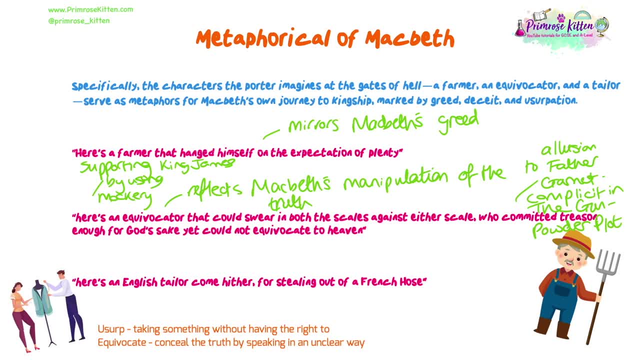 clothes fit you, And the porter also refers to a tailor. So the tailor steals materials to fashion himself. That's why it says: here's an English tailor, come hither for stealing our French hose. And the porter also refers to a tailor. so the tailor steals materials to fashion himself. 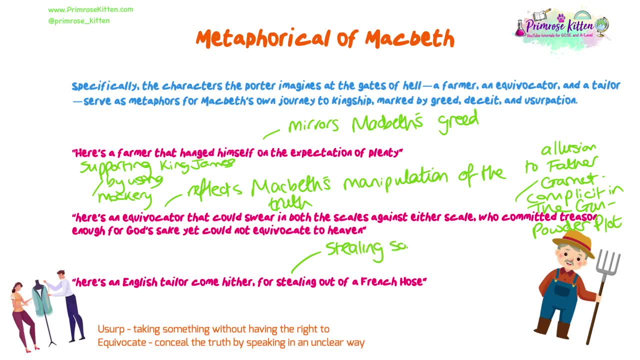 And the porter also refers to a tailor. so the tailor steals materials to fashion himself And the essentially this symbolises Macbeth's theft of the throne and the titles that were not rightfully his. So all of those figures together encapsulate the sins that lead to Macbeth's downfall. 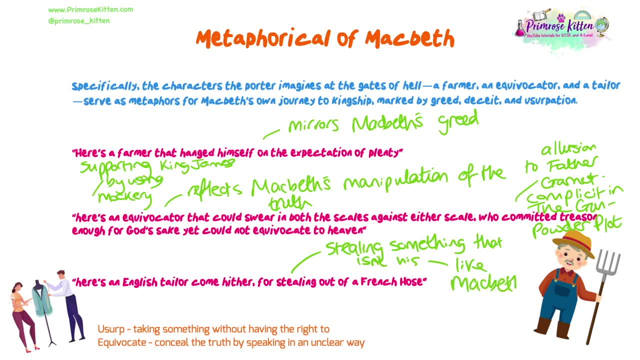 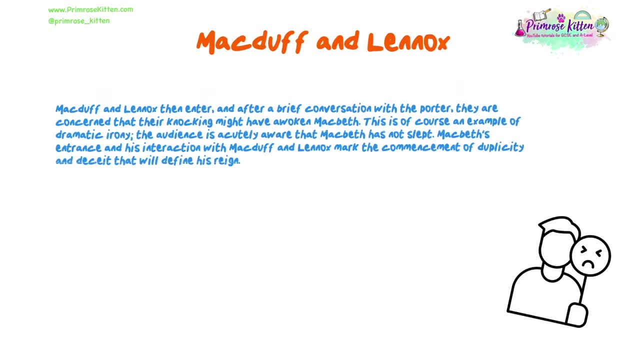 emphasising the theme that such transgressions inevitably lead to moral damnation. Now, Macduff and Lennox then enter and after a brief conversation with the porter, they are concerned that their knocking might have awoken Macbeth. This is, of course, an example of dramatic 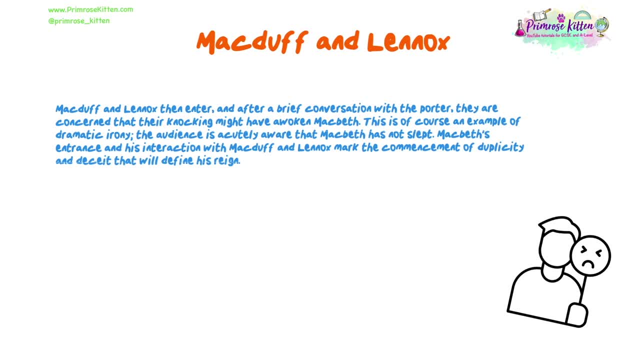 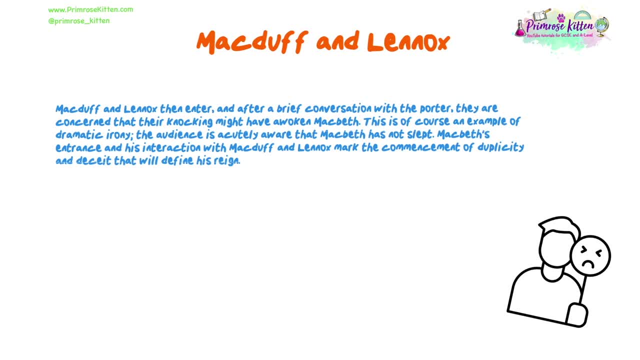 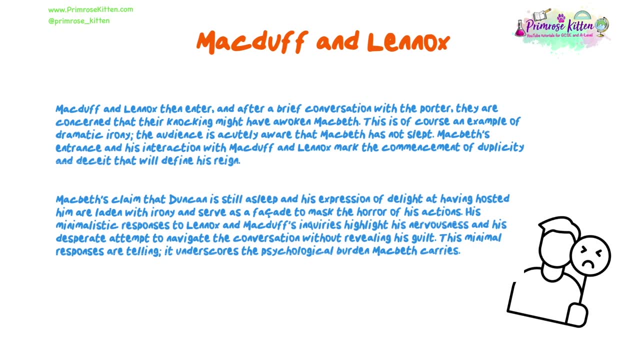 essentially defines his whole reign as king Macbeth's claim that Duncan is still asleep and his expression of delight at having hosted him are laden or full of irony and serve as a façade to mask the horror of his actions. His minimalistic response to the fact that he is still asleep is: 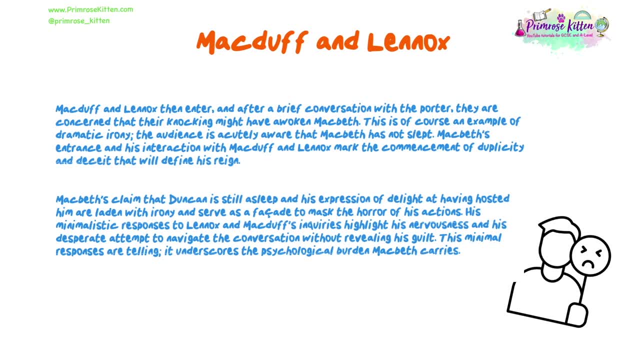 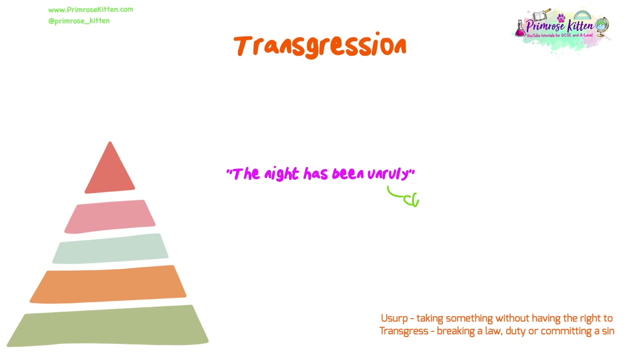 to highlight his nervousness and his desperate attempt to navigate the conversation without revealing his guilt. The minimal responses are telling. it underscores the psychological burden Macbeth is carrying. As the conversation continues, Lennox observes that the night has been unruly, and that's just essentially saying the night has been very chaotic, and introduces a motif that 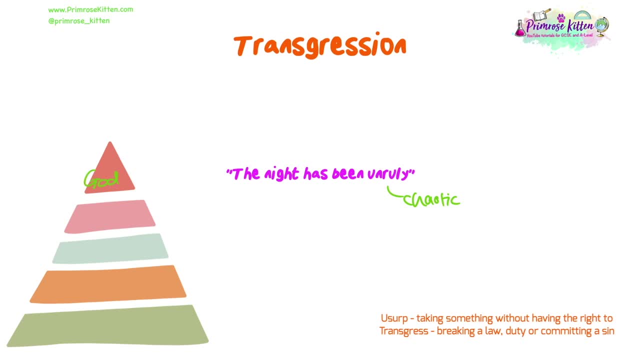 resonates deeply with the audience. The night has been very chaotic and it introduces a motif that resonates deeply throughout the play: the disruption of the natural order. His description of the earth as feverous and shaking is a potent metaphor for the societal and supernatural disarray that's been 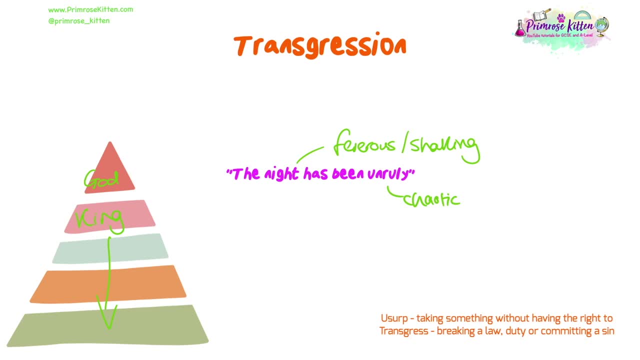 triggered by Duncan's murder. This imagery essentially aligns with the Elizabethan and Jacobean concept of the great chain of being and that's a hierarchical structure that I'm sure you know of. The hierarchy positions that kings divine right to rule are something that creates harmony. 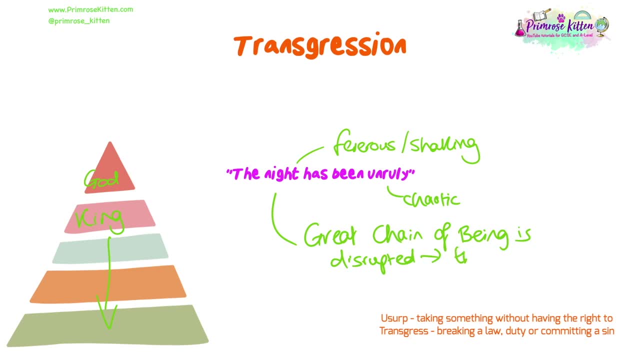 because that structure is as it should be, and if this structure is disrupted, there is going to be chaos. Macbeth's usurpation of the throne then therefore represents not only something that isn't actually his, but a dangerous violation of the natural and divine order, leading to chaos both. 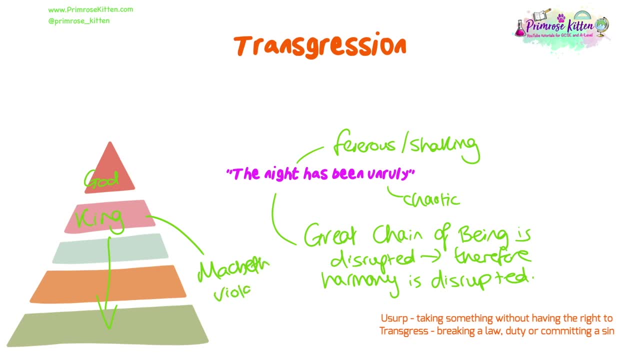 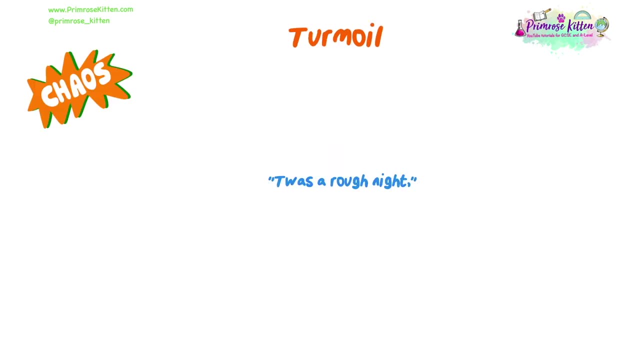 in the human world and in the natural world as well. Macbeth's brief response to A Rough Night, while seemingly insignificant, carries weight in the context of Lennox's earlier remarks. His attempt to downplay the events of the night is a strategy to deflect attention from himself, but it also 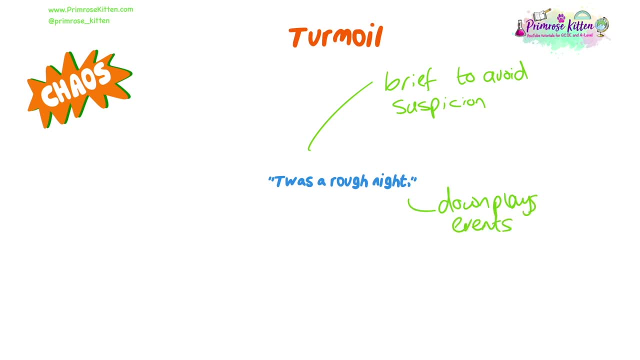 signals his acknowledgement of the upheaval his actions have actually caused. So here the use of dramatic irony, the start of Macbeth's duplicity and the imagery of a world thrown into turmoil encapsulate the tragic downfall of Macbeth and his reign. 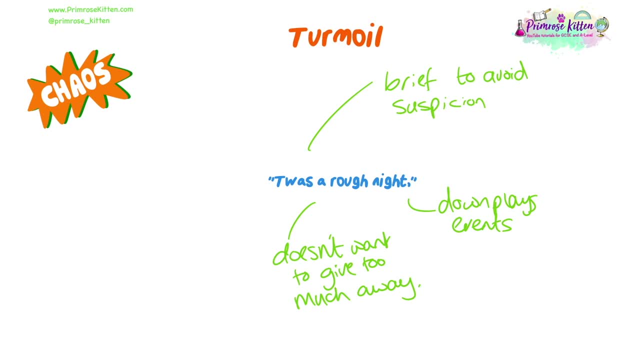 The murder of Duncan is not just a crime against the king. it is a disruption to the very fabric of the universe, setting in motion a chain of events that will lead to societal collapse and personal damnation for Macbeth. So what he has done is huge and he will be punished for it. these are all signs. 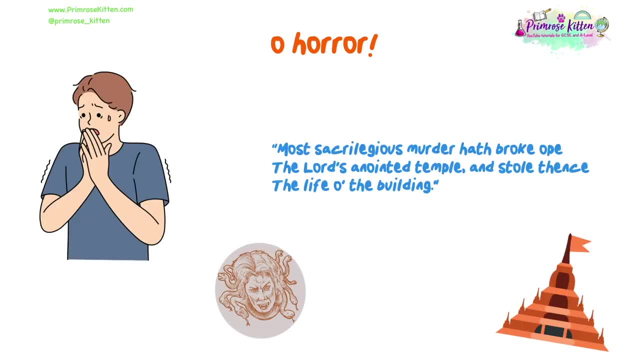 that that is coming Now. don't forget: nobody has actually discovered the body yet. the only people that know of Macbeth are Lady Macbeth. This speech is a critical point now because Macduff discovers Duncan's murder and his initial. 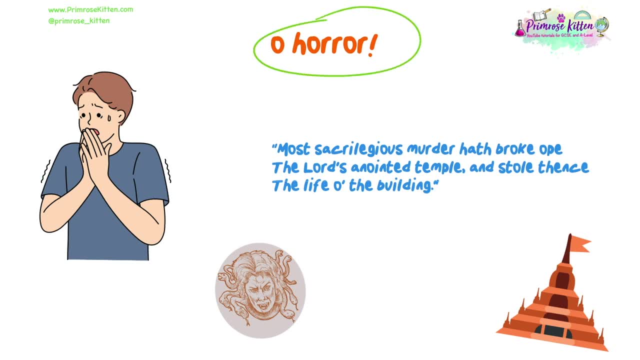 reaction is literally just to shout: oh, horror, horror, horror. and he also says: tongue nor heart cannot conceive nor name thee. so it captures this real, indescribable shock and despair that such a sacrilegious act has been permitted where Duncan should have been safe and he actually 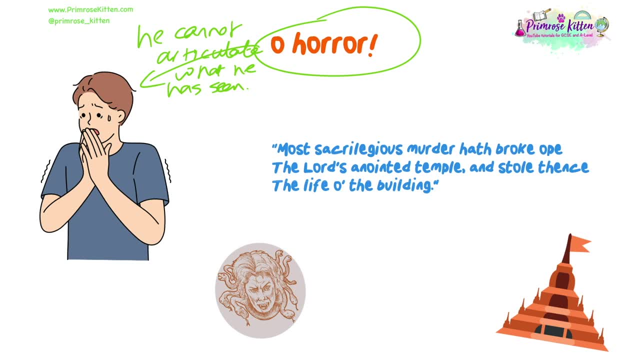 can't articulate, or in other words speak about the scene's gruesomeness, and that signals to the audience the horrific nature of the transgression that has taken place. He is absolutely horrified because it shouldn't happen. Macduff's description of Duncan's murder as the destruction of the 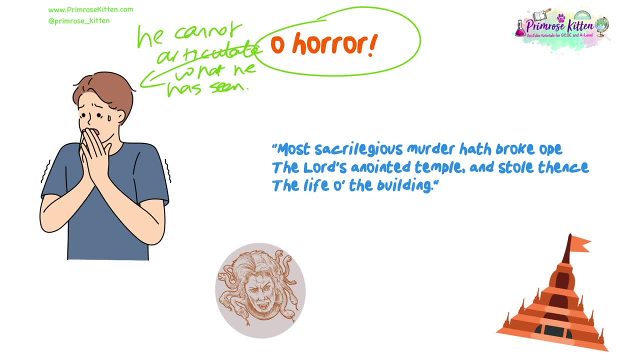 Lord's anointed temple further supports the notion of the divine right of kings, with the king's body symbolically representing this holy structure like a temple. This violation is not just against the human Duncan, but against God's appointed ruler on earth as well. 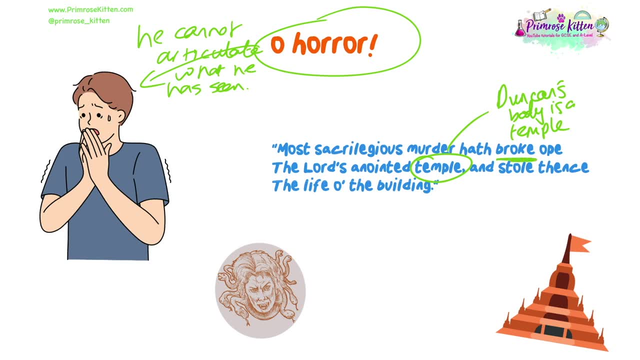 So in the Jacobean context, this comparison would have resonated deeply, with the audience affirming the gravity of regicide or just, in other words, showing how big this disaster is going to be, because it was not only a political crime but also a spiritual. 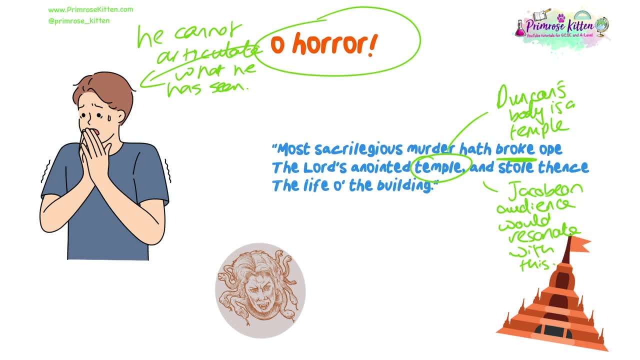 one as well, an act that ignores how sacred the monarch was at the time. Now, the others almost don't want to believe Macduff, and so he advises them- this is a quote- to approach the chamber and say that this is the end of the world. this is the end of the world. this is the end of the world. 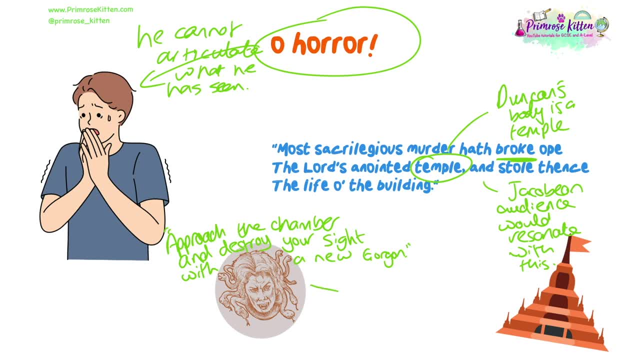 And the allusion to a mythological creature, a gorgon, whose gaze can turn men to stone, amplifies the scene's horror. The image of a gorgon serves as a powerful metaphor for the monstrous nature of the act, indicating that the sight of Duncan's slain body has a petrifying 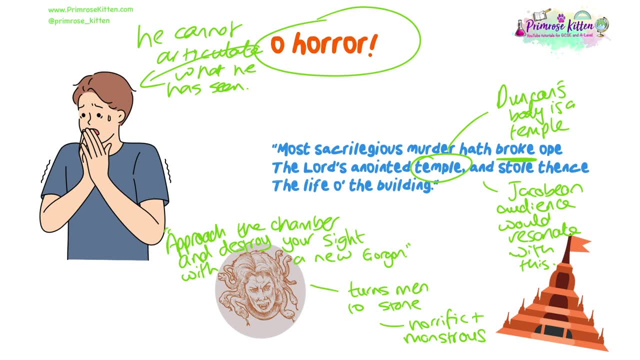 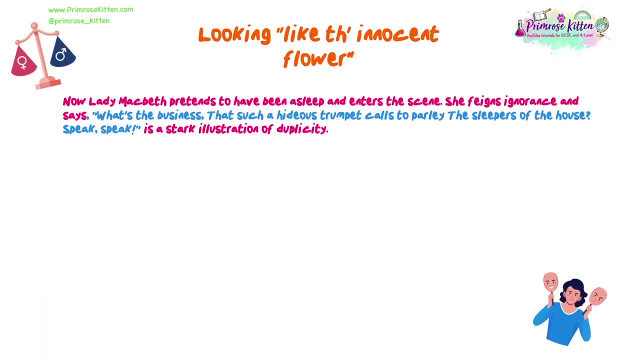 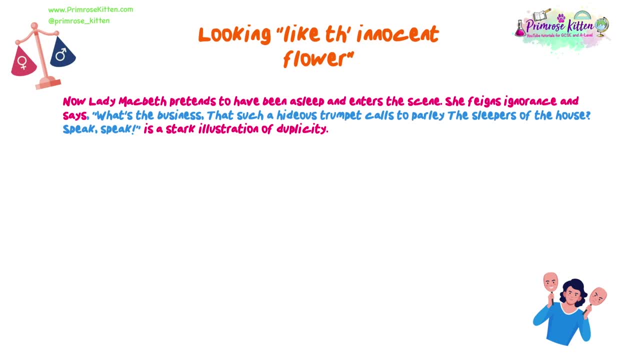 And enters the scene. She feigns ignorance, and that just means she pretends to be completely unaware. If you feign something, you fake it, And she says: what's the business that such a hideous trumpet calls to parley? the sleepers of the house Speak, And this is a stark illustration of duplicity. 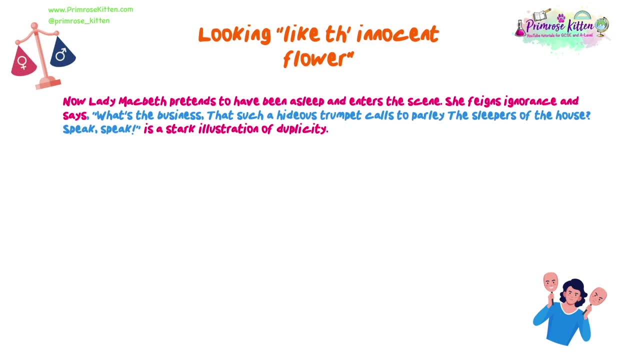 And duplicity just means being two-faced. That's what that little picture is down there in the corner. She pretends to be angry that there is such a commotion. Her performance of innocence amidst the chaos that she helped to orchestrate is a prime example of the theme of appearance versus reality. 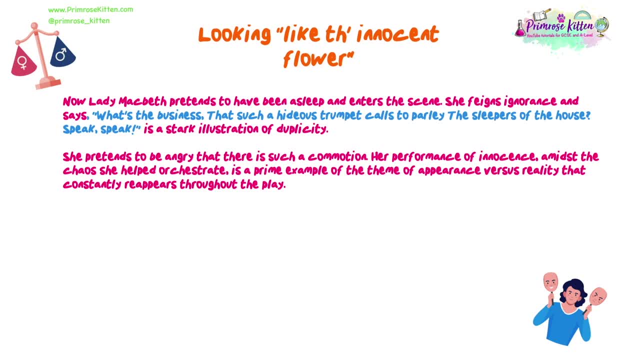 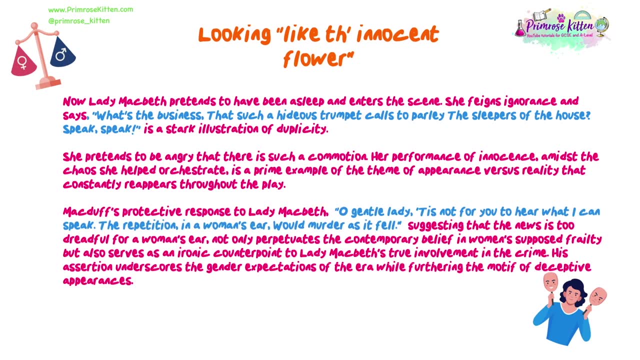 that constantly reappears throughout the play, Macduff's protective response to Lady Macbeth: oh, gentle lady, it is not for you to hear what I can speak. The repetition in a woman's ear would murder as it fell suggests that the news is too dreadful for a woman's ear. not only perpetuating 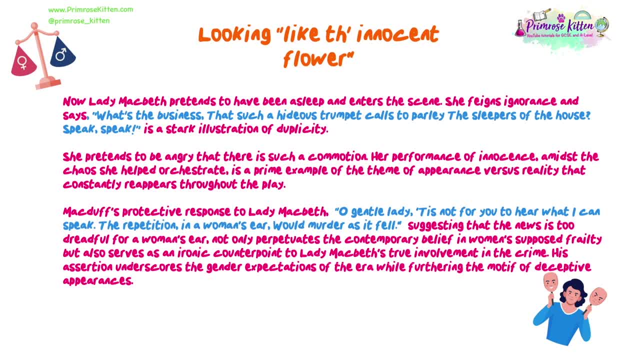 the contemporary belief in women's supposed frailty and weakness, but it also serves as an ironic counterpoint to Lady Macbeth's true and true self. Macduff's assertion underscores the gender expectations of the Jacobean era. while furthering the motif of deceptive appearances. She can use her femininity to appear innocent and 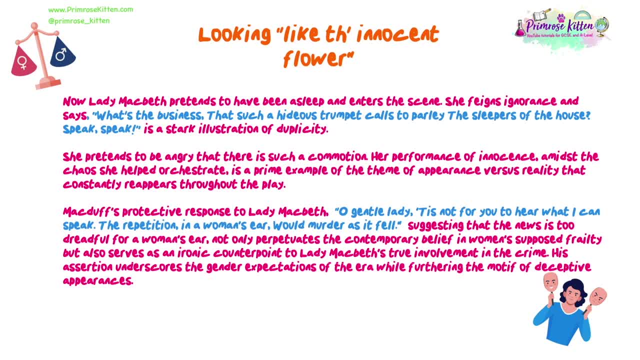 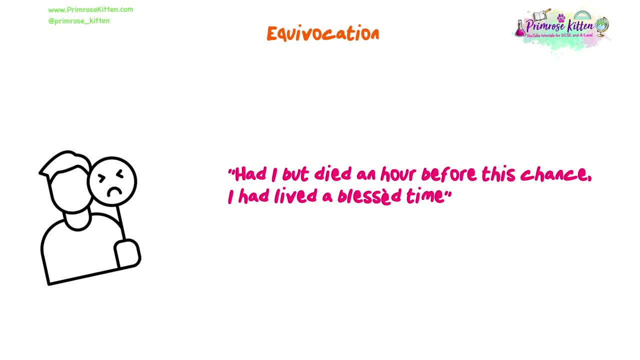 weak and vulnerable, and it works really really well for her in this moment. Now, obviously, the panic continues and Macbeth expresses this wishful thought: Had I but died an hour before this chance, I had lived a blessed time time, and this carries a really kind of sly and sneaky double meaning to the unaware, the people. 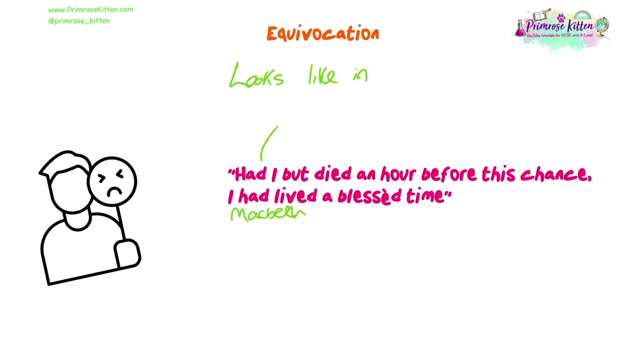 surrounding him. it reflects a nobleman's sorrow for his king. he's grieving, he's really distraught. he wishes that he didn't have to live in a world without Duncan in it, and if he died an hour ago he wouldn't have to. but then also you've got this kind of more subtle, sneaky reveal from Macbeth as 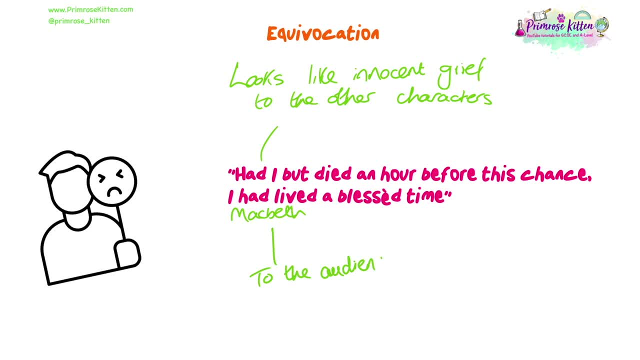 well, so to the audience it actually reveals Macbeth's inward torment and the realization that his soul is now eternally stained with regicide's guilt. so if he could have died an hour ago he would have never felt this guilt. so that's the kind of double meaning there, and it 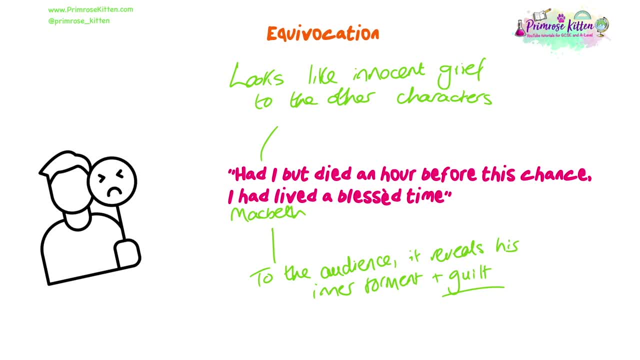 captures Macbeth's duality, or in other words the two sides to him as both the mourner, the griever and the murderer, and that's a mantra- between his ambitions and the devastating consequences of his actions. this is actually another example of equivocation as well, because he cleverly speaks. 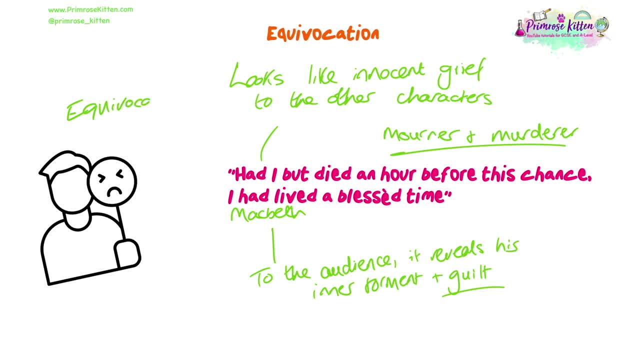 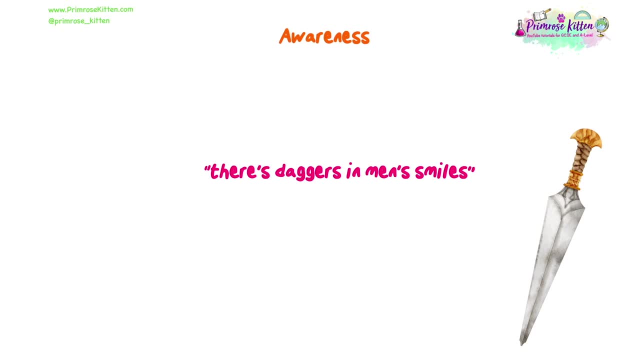 his true feelings, but in a way where nobody's going to suspect him. now, at the end of this extremely tense scene, the sons of Duncan, Malcolm and Donalbine are seemingly very aware that somebody is lying around them. Donalbine says there's daggers in. 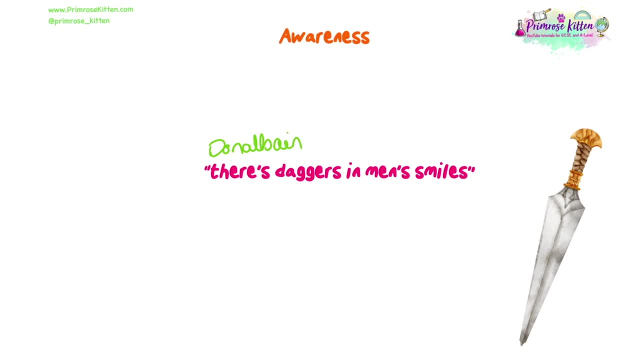 man's smiles, and this evokes a powerful image of concealed malice, revealing a landscape where appearances are deceiving and trust has been compromised. he can't trust anyone around him. the use of the noun daggers captures the brutal and sinister nature of deception. a dagger is a weapon that requires closeness. to commit a murder, obviously you have to be a lot. 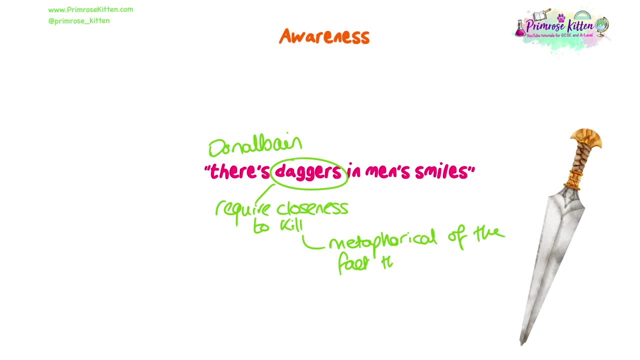 closer than if, for example, you were using a sword. so it suggests that someone close to Duncan has committed this murder and conceals it with a smile. now they are clearly not as naive as their father who, in act one, scene four, said there's no art to find the mine's construction in the face. 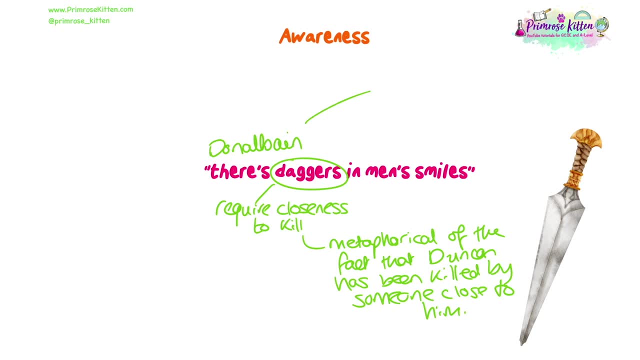 that was about the betrayal of the original Thane of Cawdor, and now he's let another one do it to him. So it suggests that Malcolm is a lot more aware, and he would make Eamon potentially a more stable king, as he doesn't trust people as easily as his father did. And their decision then to flee to 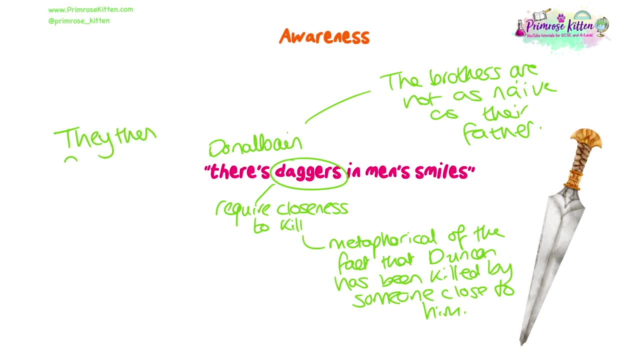 England and Ireland encapsulates a survival instinct and an acknowledgement that the court around him is now a den of liars, potential assassins, but it does, however, make them look guilty too. The others actually kind of blame them for bribing the two guards, and that's why. 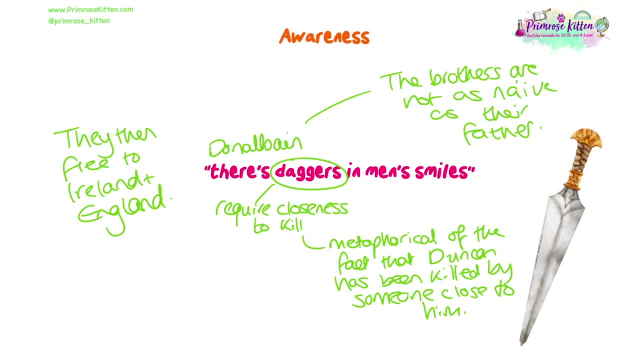 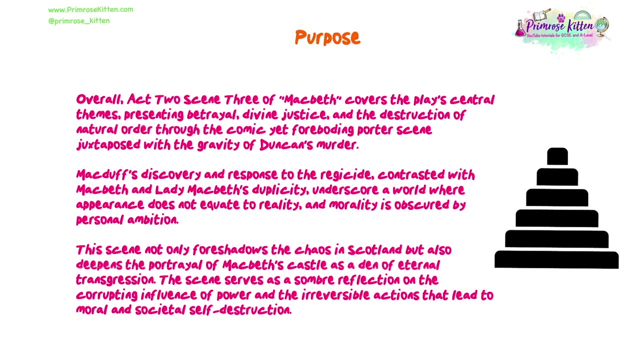 they've run away, So it doesn't really help their cause, but obviously they're doing it for their safety. Now, overall, Act 2, Scene 3 of Macbeth covers the play's central themes, presenting betrayal, divine justice and the destruction of natural order, through the comic, but also 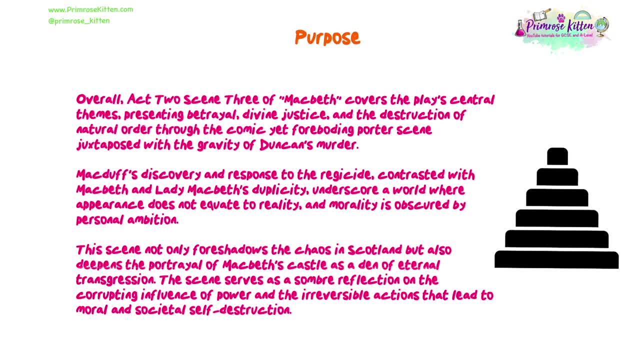 foreboding portisine juxtaposed with the gravity of Duncan's murder, Macduff's discovery and response to the murder is a bit different. Macduff's discovery and response to the murder is a bit the regicide contrasted with Macbeth, and Lady Macbeth's duplicity Underscore a world where 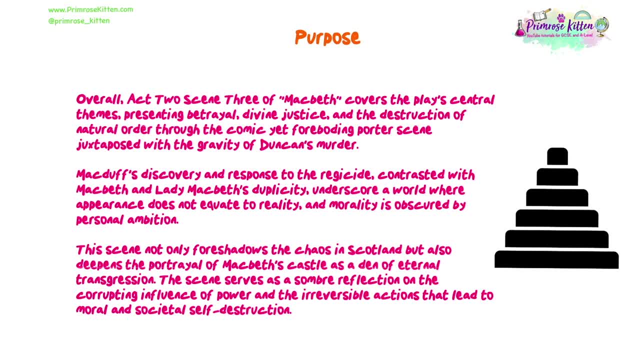 appearance does not equate to reality and morality is obscured by personal ambition. This scene not only foreshadows the chaos in Scotland, but also deepens the portrayal of Macbeth's castle as a den of eternal transgression, and the scene serves as a really sombre reflection. 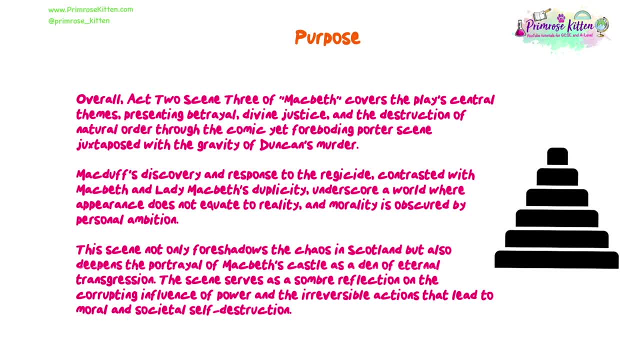 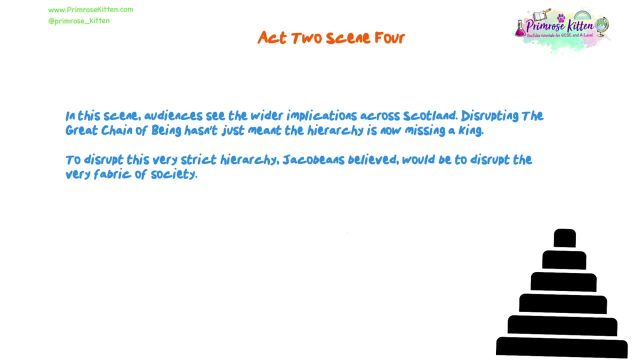 on the corrupting influence of power and what it's done to Macbeth, essentially, and the irreversible actions that lead to moral and societal self-destruction. Now, as I said, I've kind of combined Scenes 3 and Scenes 4 as a whole video because I wanted 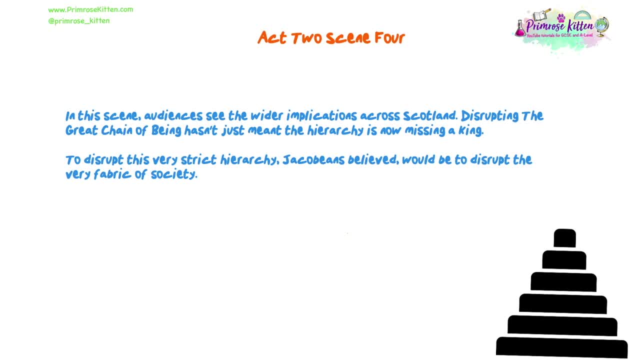 to show the immediate aftermath. So in both scenes you can see the immediate turmoil that follows the murder of Duncan, and in this one especially it shows the wider implications across Scotland. Disrupting the great decline of being hasn't just meant the hierarchies now. 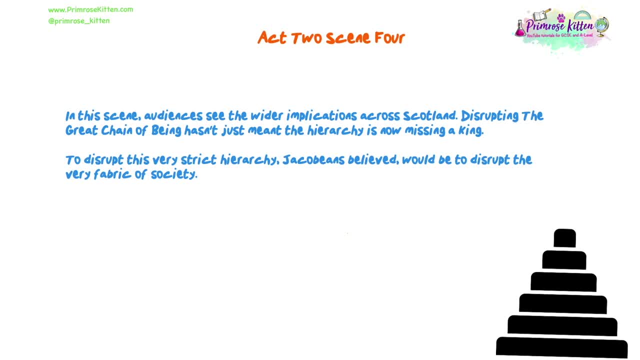 as we said before, disrupting this very strict hierarchy Jacobeyans believed would be to disrupt the values and the values of the press of current dictatorship, And that's simply not working. So I see no donation from theона mape, whose Ingham group has produced the sourcelaw for last semester's. 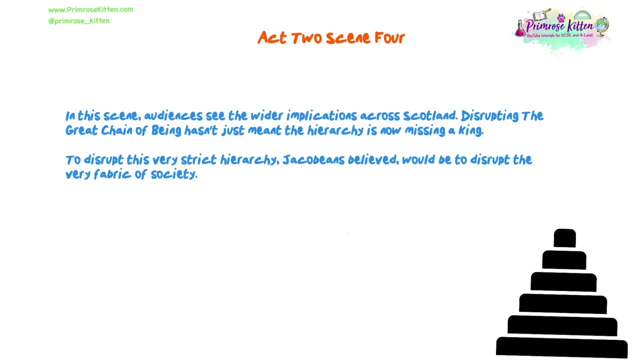 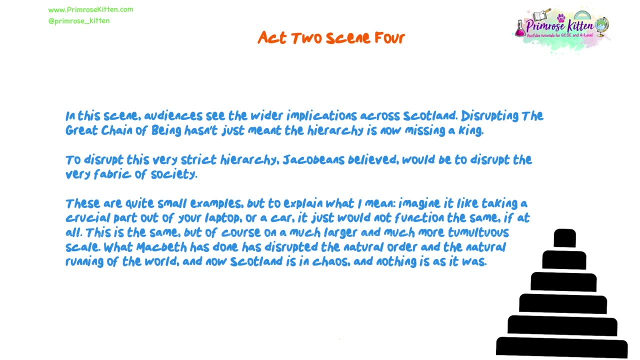 very fabric of society. So I want you to kind of imagine. these are quite small examples, but to explain what I mean, imagine it like taking a crucial part out of your laptop or a car. it just would not function the same, if at all. and this is the same, but of course on a much larger and much 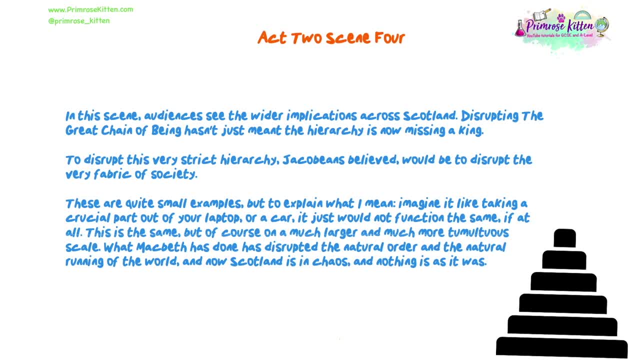 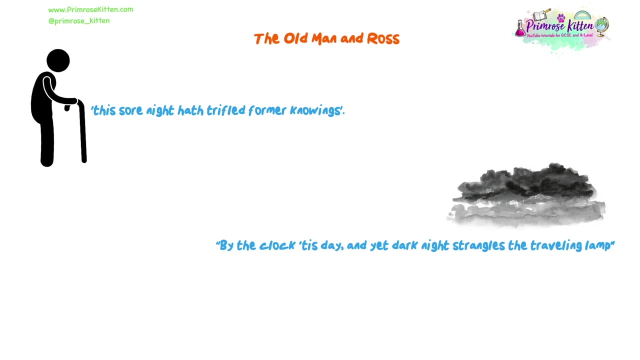 more tumultuous scale. What Macbeth has done is disrupted the natural order and the natural running of the world, and now Scotland is in chaos and nothing is as what it was before. Now, as a little summary in this scene, Act 2, Scene 4,, an old man and Ross, another Thane, discuss the 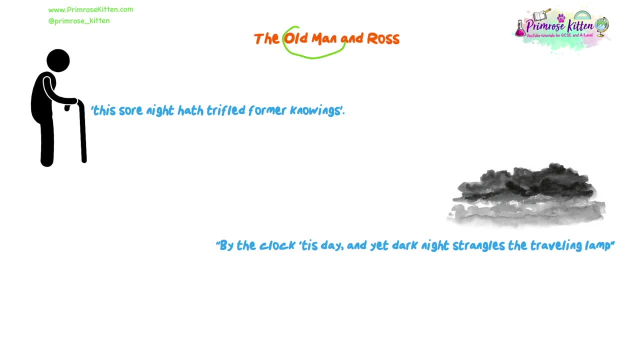 strange things that they have noticed following the death of Duncan and actually some things before it too. So Shakespeare includes this old man, which we could call a stock character, which is like a typical character you might see throughout lots of films and books: An old man. 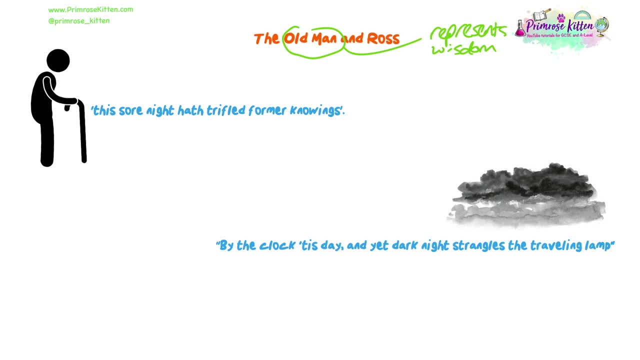 typically represent wisdom. so in literature, older characters offer wisdom to younger ones. you can imagine Dumbledore and Harry Potter, for example, and it's the same here. So the old man says that what he has seen hath trifled former knowings. so in other words, what he has known throughout his whole life is: 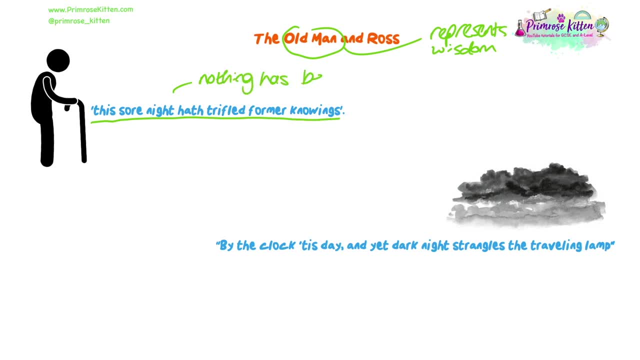 nowhere near as horrifying as what he had witnessed last night. Ross responds saying that by the clock it is day and yet dark night strangles the travelling lamp. So in other words, he's saying that it should technically be daytime and technically is daytime, but the darkness. 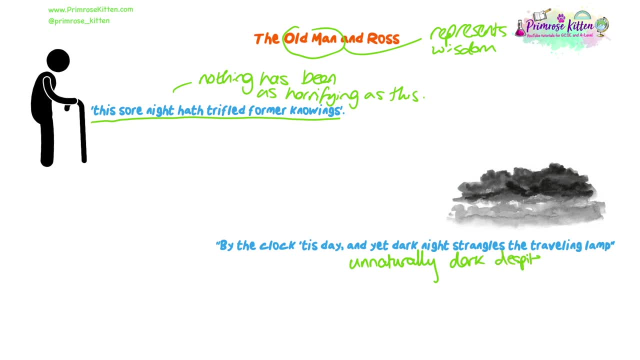 is kind of personified to be strangle in the sun, and so therefore it appears to be unnaturally dark for this time of day. And if we're going to zoom in here, we might look at the verb strangles. that's a barbaric and murderous word and it conjures images of an attack. 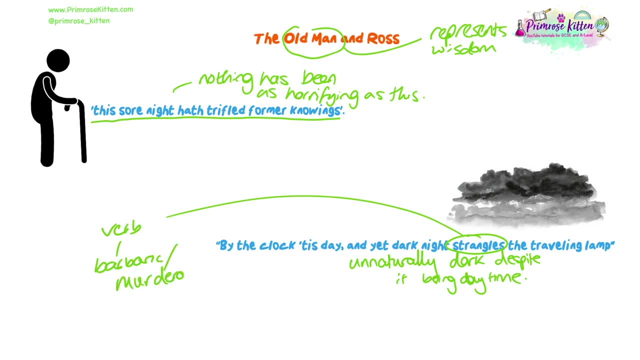 so this is, of course, representative of the attack on King Duncan. Furthermore, just as the sun provides light and life to the world and has now been extinguished by darkness, Duncan, as God's representative on earth, cannot provide light to his subjects anymore either, because he has been extinguished by something dark, in this case. 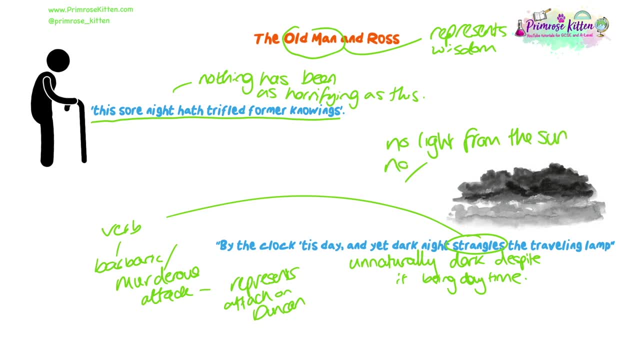 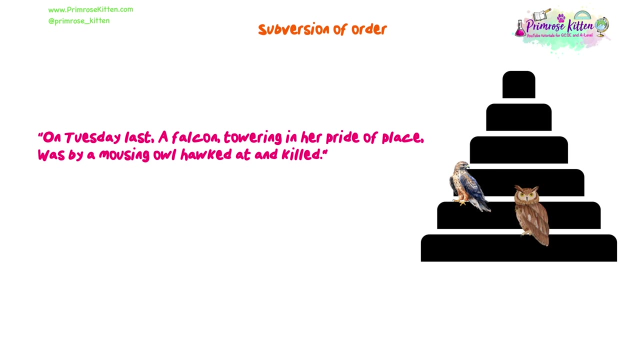 Macbeth and on a wider scale. it is symbolic of all things natural and rightful being taken from the earth. The old man agrees that it is unnatural, even like the deed, which reaffirms the audience's belief that the murder of a rightful person is not natural. So he's saying that the murder of a 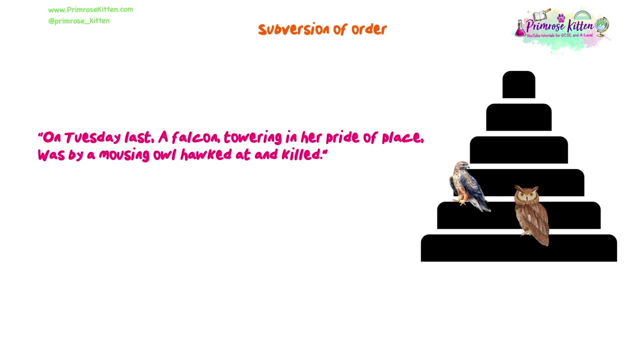 rightful king is unnatural. He continues to point out strange and unnatural events. so he says: on Tuesday last a falcon towering in her pride of place was by a mousing owl hawked at and killed. Now a falcon, as a predatory bird, should of course not be killed by an owl, but think metaphorically. 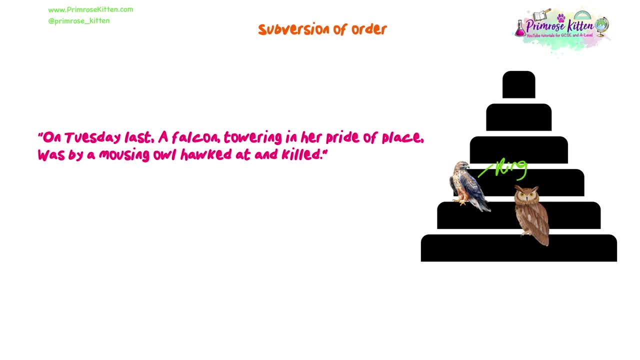 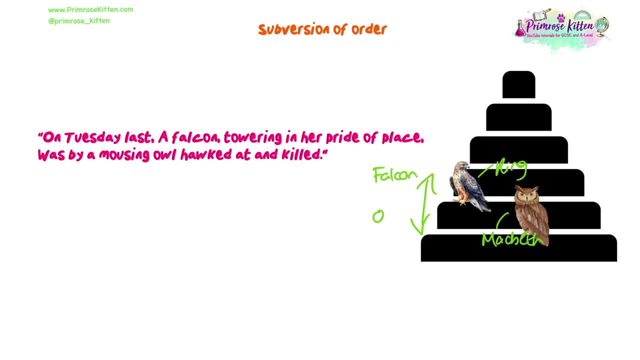 So an owl's place would be lower than a falcon's, echoing Macbeth's place as lower than King Duncan's. It shows a complete subversion of what is natural about the world, all because of what Macbeth has done, once again. Now, one thing I actually realised is that this quotation says: 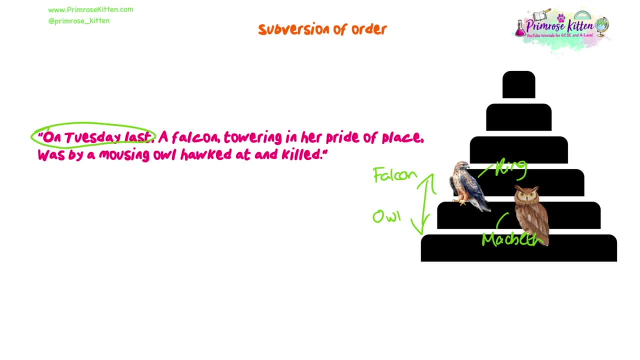 on Tuesday last. he saw this occur, but mentions the murder was only last night, So at the time he noticed it the murder would not yet have taken place, but already unnatural things were occurring. So it's almost as if Shakespeare was suggesting that God's omniscience, or in other words the 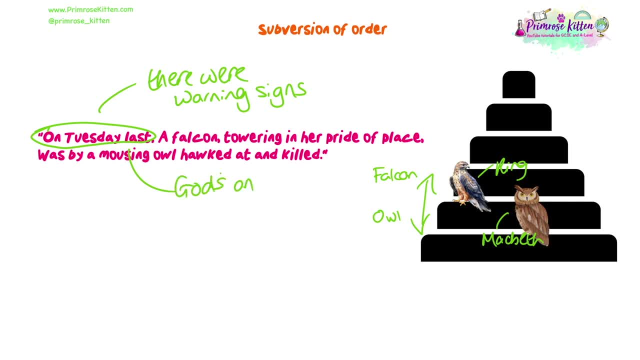 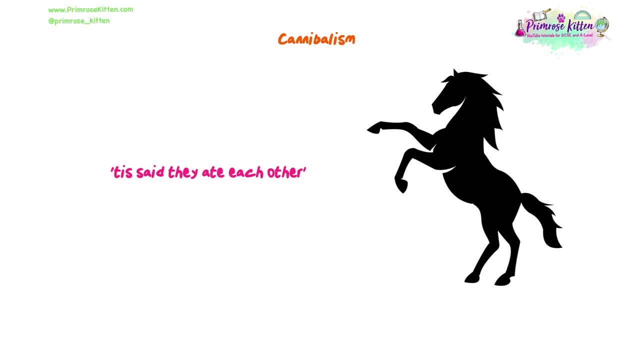 fact that he knows everything cannot be underestimated. Perhaps he knew and these were the warning signs for the people in Scotland. Finally, another interesting image I wanted to point out is the fact that Ross mentions Duncan's horses turned wild, to which the old man responds: tis said they eat each other. Now the animals have. 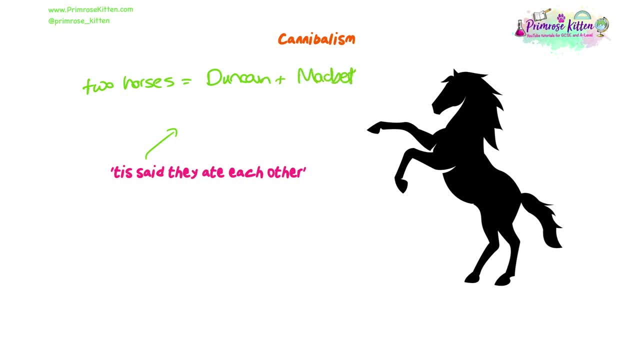 become cannibalistic, which is again very unnatural. We could see this in two ways. so first that metaphorically the two horses represent Macbeth and Duncan, the murder of his fellow man. or we could see it as not only that nature is destroyed because of what Macbeth has done, as we've seen. 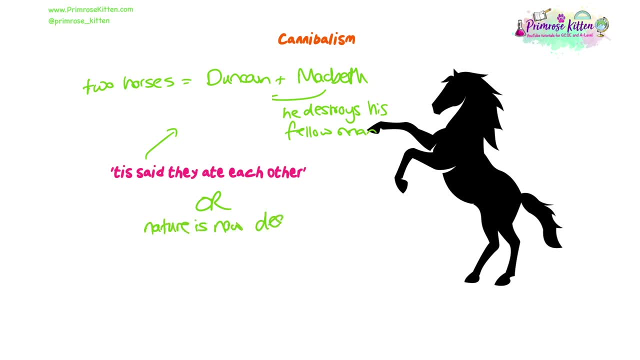 with the previous images that we've just looked at, but that now nature is also destroying itself. So, as we said, the very fabric of society is being disrupted, and this is possibly the most ominous image of all of them if we view it through the lens of that second interpretation. 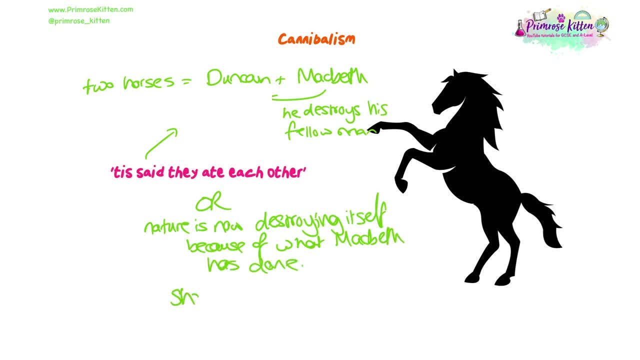 the idea that nature is now destroying itself because of what Macbeth has done. So Macbeth, by disrupting the great chain of being, has destroyed the natural order around him, but so much so that nature has now turned on itself And this image again serves as a terrible reminder of the wide-spreaded nature of society. So this is a very interesting image, and I think that's going to be a really interesting piece of work for us in terms of how we're going to continue this analysis. I hope you'll be happy about that. So now we're going to move on to